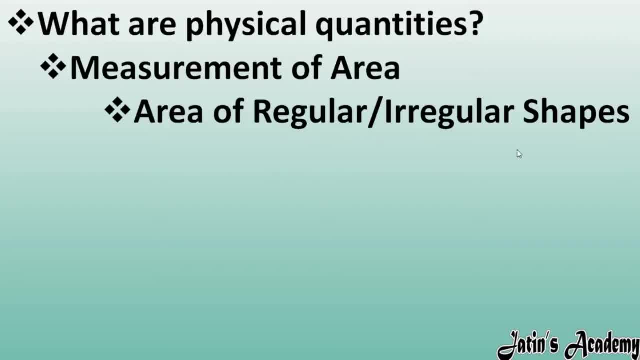 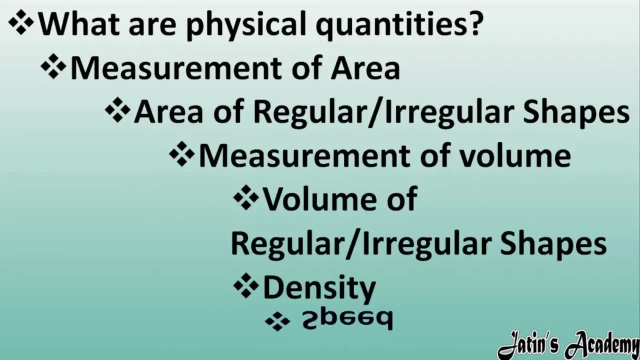 of area. Third area of regular or irregular shaped objects, Then measurement of volume, Then we will cover volume of regular or irregular shapes, Then density, And then, at last, we will cover the topic speed. So now let us start with the first topic. First topic: we 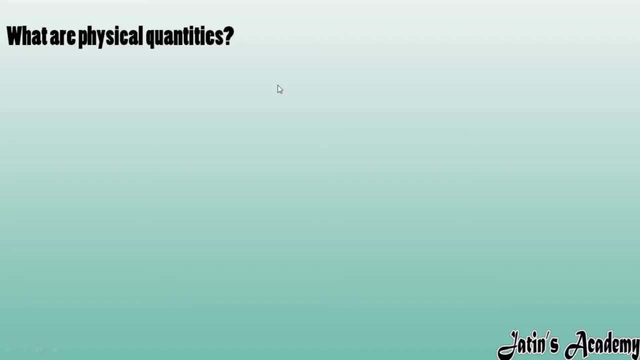 are having. what are physical quantities? So first of all, as the name suggests, physical quantities and measurement. So we should know what are physical quantities. So see the definition. what are physical quantities? Quantities that can be measured are known as physical quantities. Any quantity. 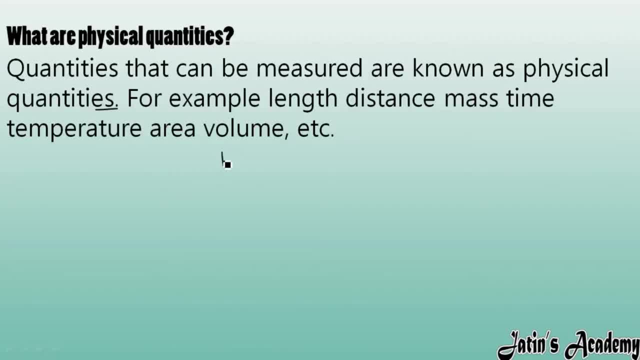 which we can measure. For example, I am having here length. This length I can measure, for I am just taking the scale and by using the scale I am going to measure the length. So the quantities that we can measure are known as physical quantities, like length I can measure. 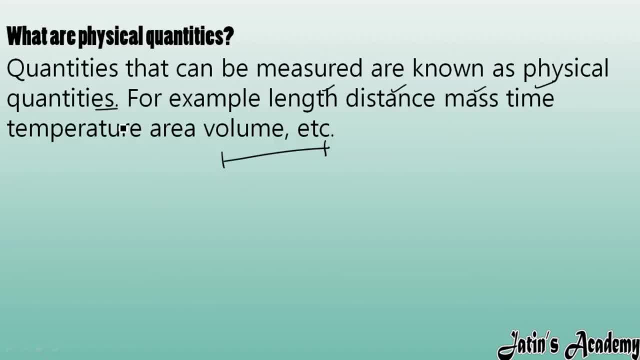 distance, I can measure mass, time, temperature, area, volume, etc. So whatever quantities are there that we can measure are known as physical quantities. So like this we can see many instruments are there, For example with this instrument. 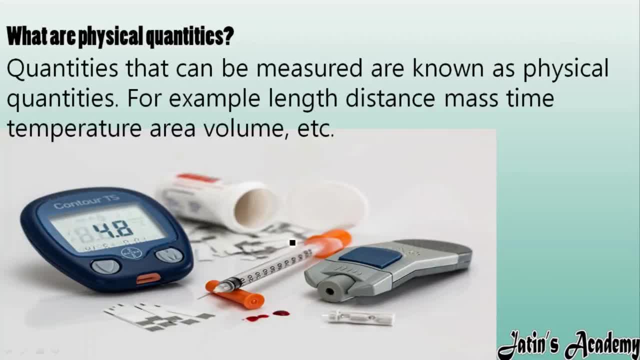 we can measure the time With this instrument. we can measure the like blood. We can see how much blood is present in our body. So range is there. So many instruments are there to measure different physical quantities. So the physical quantities are the quantities. 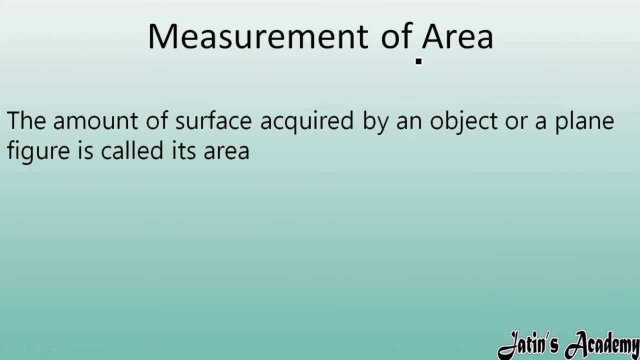 that can be measured. Next we are having measurement of area, So first of all we should know that how we can measure some physical quantities. There are some instruments by which we can measure different physical quantities and one by one, we are going to. 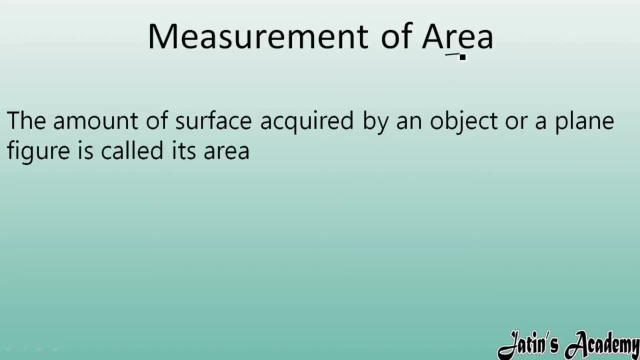 study about that also. So first we are having measurement of area, that how we are going to study the or how we are going to measure the area. So before this we should know what is an area. So what is an area? The amount of surface acquired by an object. Amount. 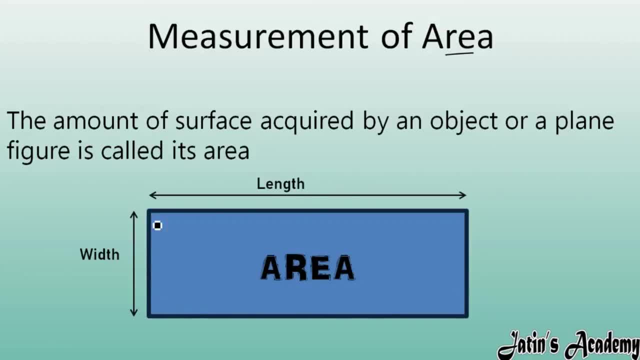 of surface acquired by any object or any plane figure. that is known as its area. So this area is having some kind of length, plus area is having some kind of width. So this amount of surface acquired by any object or the plane figure is known as its area. And next we 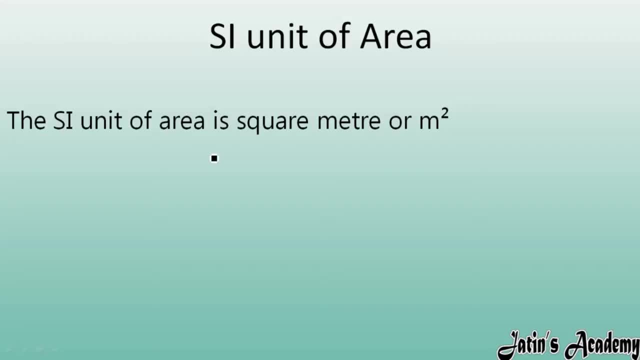 are having SI unit of area. So whatever things we are measuring, for the measurement we are always using some kind of SI units. SI unit means standard international units. What are SI units? SI units are those units which are widely acceptable. 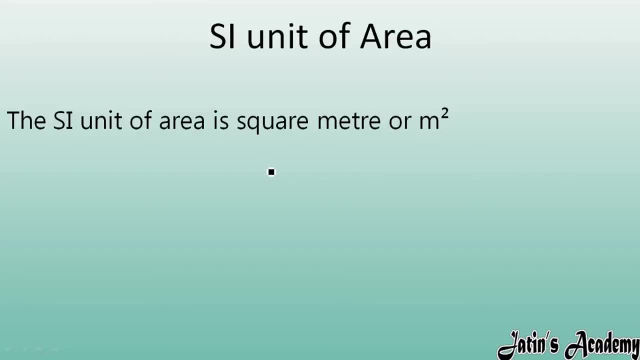 SI unit is the unit which is acceptable to all over the society. The whole society is going to accept only one unit and that unit is known SI unit system. And according to SI unit system area, we are going to measure in square meter, or you can say meter square. 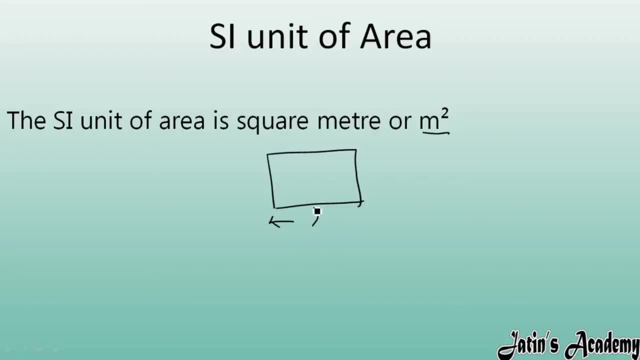 How does it? it is going to measure. For example, here I am having this area, So here in this area somewhat length is there and here somewhat breadth is there, So here length is in meter, breadth in meter. 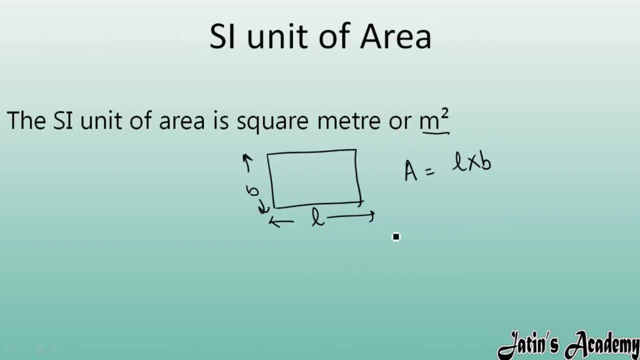 So, as we know, area, for example, this is a rectangle. Area over this, this is a rectangle. Area of rectangle is length multiply breadth. For example, this is 5 centimeter, or this is 5 meter and this is 4 meter. 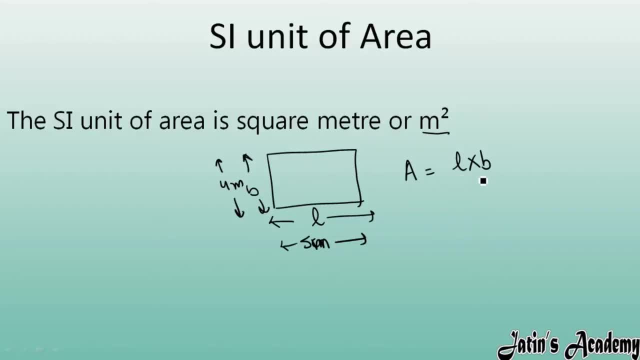 Fine. So area of rectangle must be: area is equals to length multiply breadth. So area is equals to length multiply breadth. Length is 5 meter, multiply breadth is 4 meter. So 5: 4s are 20 meter into meter, that is meter square. 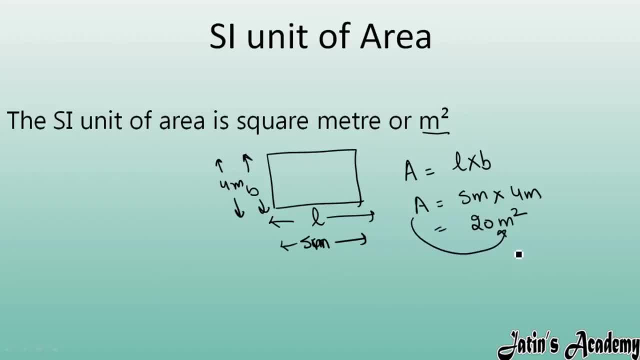 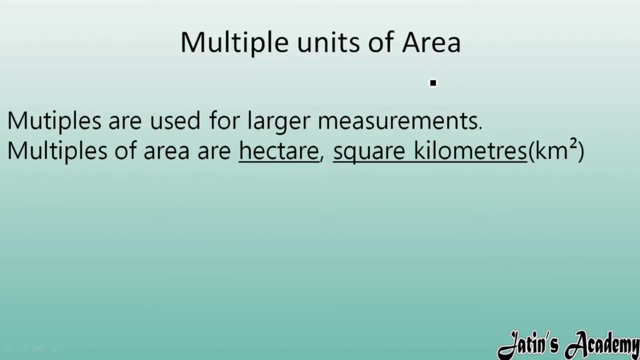 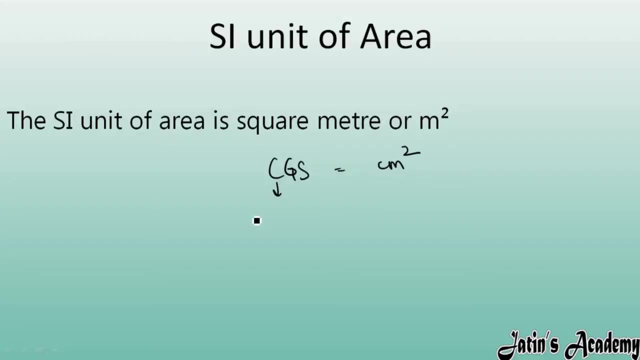 So area as a unit always is meter square. Next we are having multiples of area, like as a unit of area is meter, If you talk about the CGS unit. CGS unit of area is centimeter square. So here C means centimeter, G means gram and S means second. 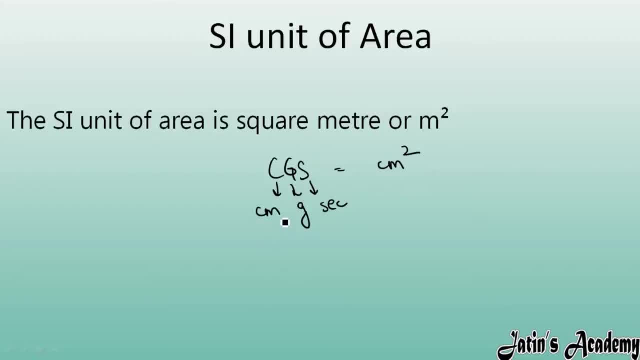 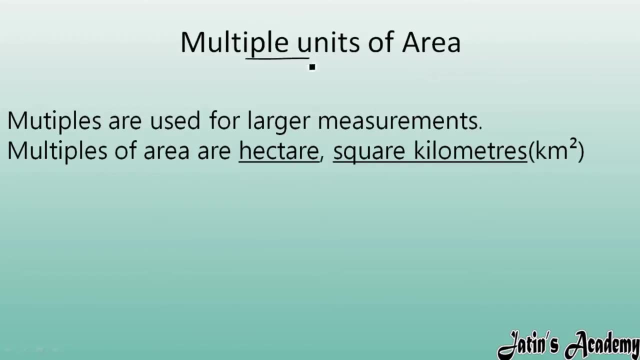 So as a unit of area- is sorry CGS- unit of area is centimeter square. Multiples unit of area. What do you mean by multiple units? Multiple unit means the units which are bigger, Means which are bigger than meter square, that areas are known as multiple units and the 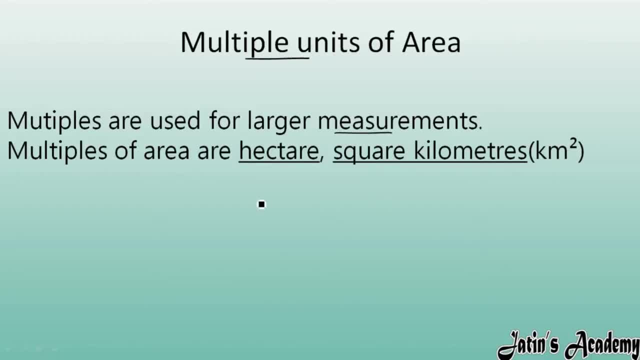 multiples are used for larger measurements. Okay So, multiples of area are hectare square kilometer. So these are some units which we are using for larger measurement of area. This is a relation between multiple units plus the S unit of area. 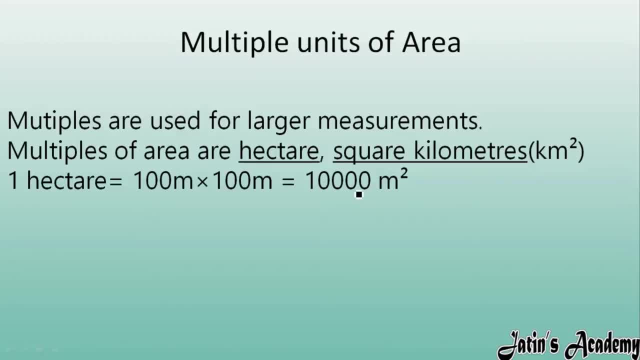 So here is a relation: 1 hectare is equals to 1,, 10,, 100,, 1000,, 10,000.. This is the relation between the bigger SI unit, bigger unit plus SI unit of the area. So multiple is hectare and here SI unit is meter square. 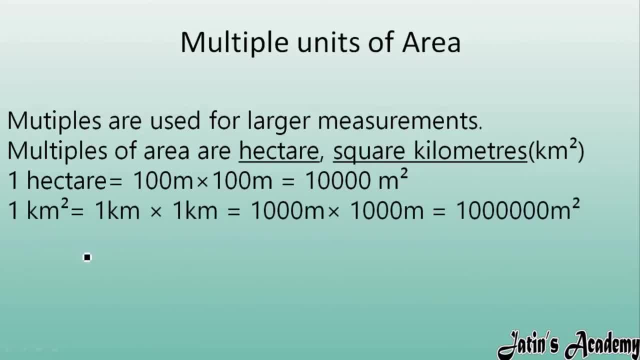 So next we are having second relationship: 1 kilometer square. Can I write 1 kilometer square as 1 kilometer multiply 1 kilometer, because it is same. only kilometer square means kilometer multiply kilometer And, as we know, 1 kilometer is equal. 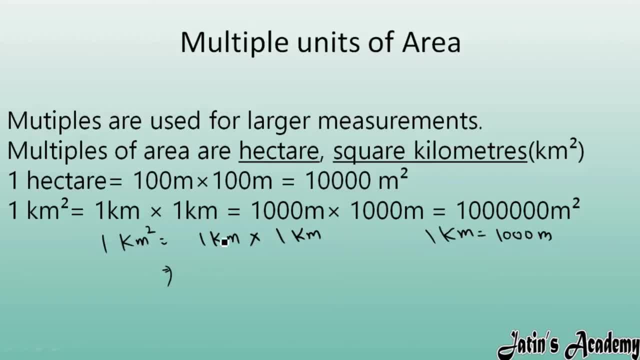 Is to 1000 meter, fine. So here can I put this value: 1 kilometer is equals to 1000 meter. So here put this value: 1 kilometer means 1000 meter. multiply this: 1 kilometer means 1000 meter. 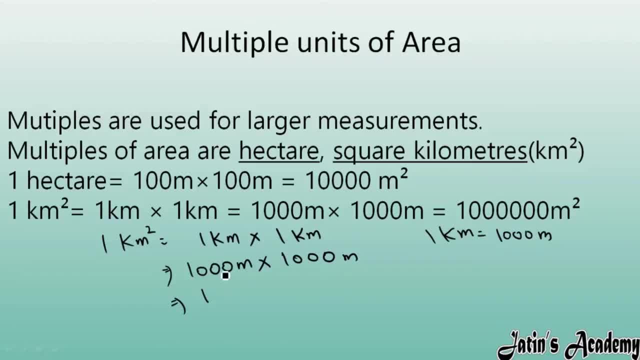 after doing the multiplication what we will get? 1 with 6 zeros meter square. So 1 kilometer square is equals to this much meter square. So this is a second relationship between the multiple unit of area with the SI unit of area. 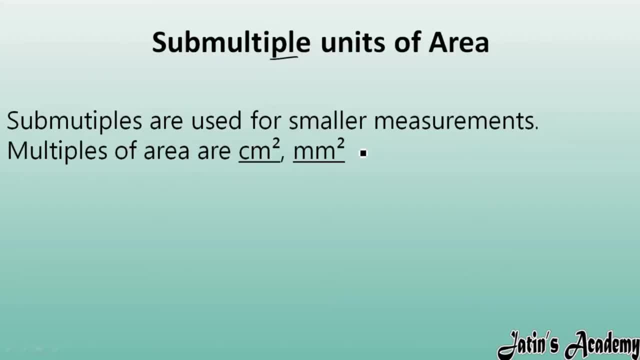 Next, we are having some multiple units of area. What do you mean by some multiple units? Some multiples are that units which we are using for smaller measurements, If you are having very small area and to measure that very small area we are not using hectare. 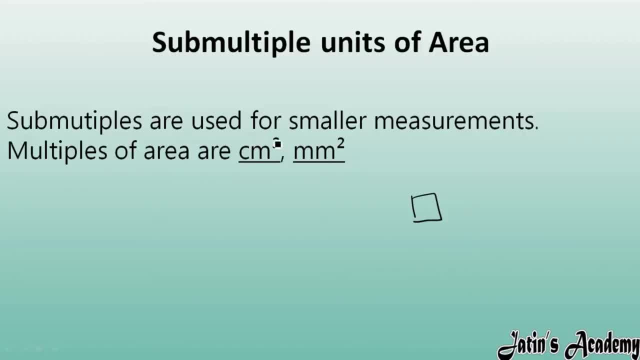 We are not using kilometer square, We are just using centimeter square or millimeter square. that we can also call it as some multiple units of area. So here we are having some relation. 1 centimeter square. Firstly, we are going to do the relationship between 1 centimeter square and meter square. 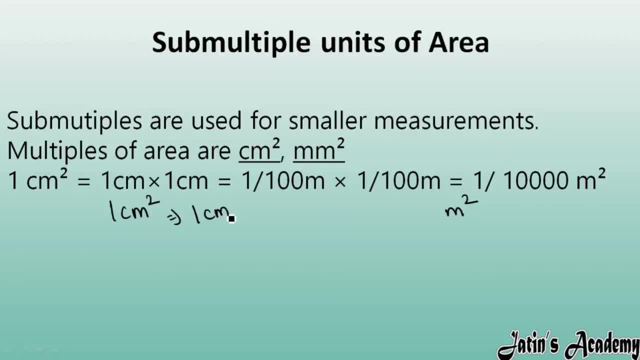 So can I write this 1 centimeter square as 1 centimeter multiply 1 centimeter, because it is same, only 1 centimeter square, So 1 centimeter is equals to 1 over 100 meter. This relation we are having between meter and centimeter. 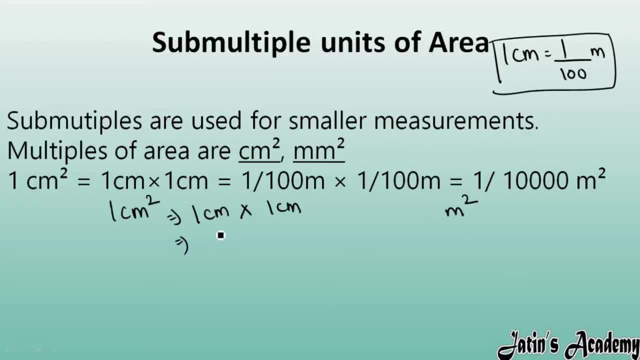 So here I am going to put the value of centimeter in terms of meter. So 1 centimeter is equals to 1 over 100 meter. multiply 1 centimeter again is 1 over 100 meter. So solve this: 1 multiply 1 is 1.. 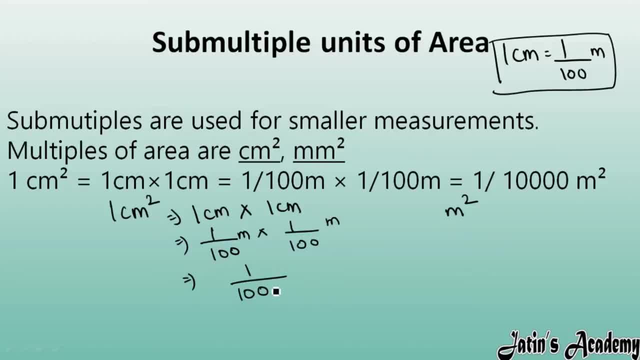 100 multiply 100 means 1.. 1,, 2,, 3 with 4 zeros meter square. So 1 centimeter square is equals to 1 by this much meter square. This you have to remember because in exams it can ask to you that what is the relation between sub multiple centimeter square and SI unit meter square? 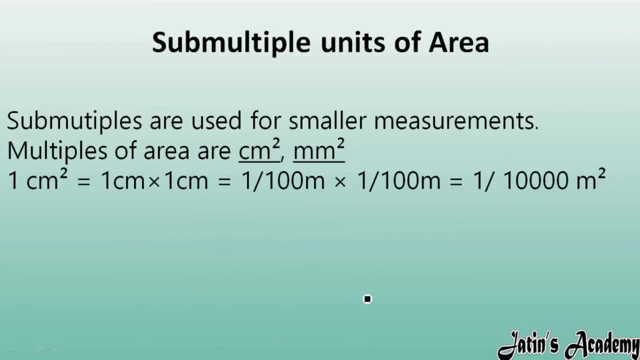 So this we have to remember. So 1 millimeter square is equals to 1 over 100 meter square. Next we are having second sub multiple: 1 millimeter square, So 1 millimeter square. can I write like this: 1 millimeter multiply 1 millimeter, and then we are having this relation: 1 millimeter is equals to 1 by 10 centimeter. 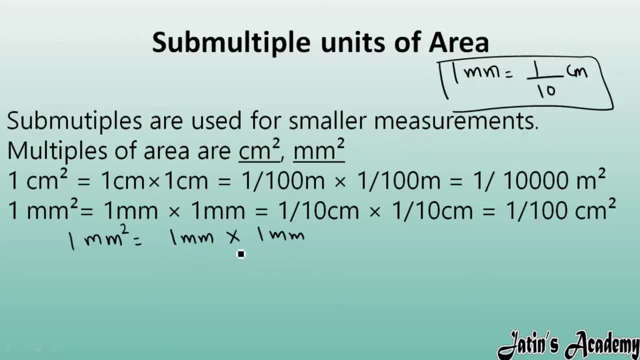 This relation you have to remember. So instead of 1 millimeter I am going to put in the form of centimeter. So 1 by 10 centimeter multiply 1 by 10.. So here, 1 multiply 1 means 1 over 10. multiply 10 means 100 centimeter square. 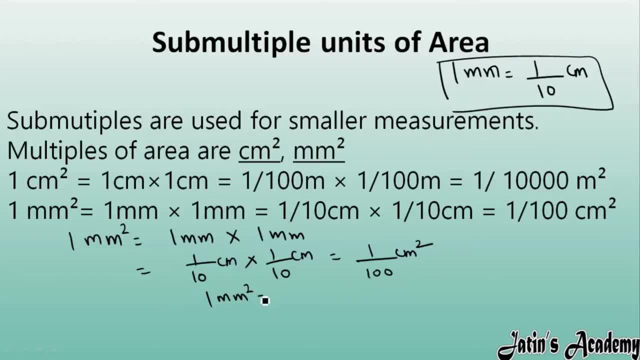 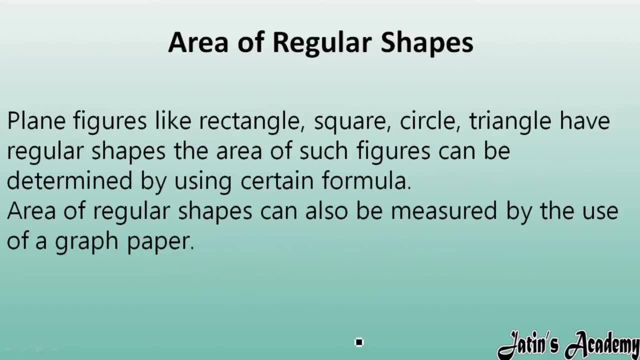 This is the relation between millimeter square: 1 millimeter square is equals to 1 by 100 centimeter square, Fine. Next, we are having area of regular shapes. Here, for example, we are having different kind of regular shapes. 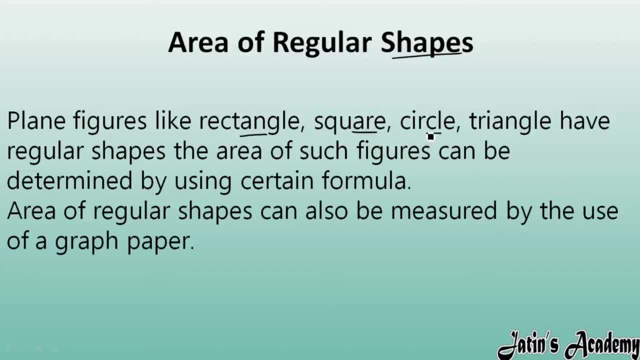 Plain figures we are having, like rectangle, square, circle, triangle. So these figures We are fixed length, is there fixed breadth? is there fixed height? is there So that plain figures are known as regular shaped objects? Fine, So how to measure the area of these regular shaped object? 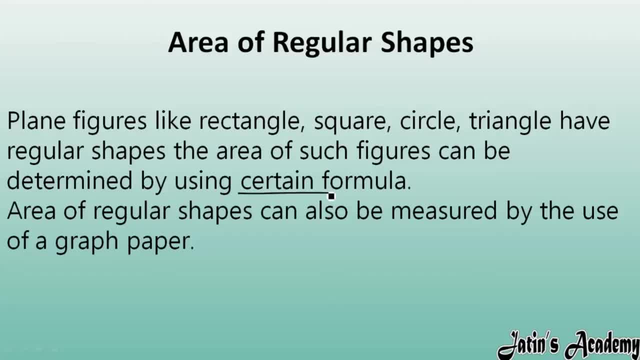 So we can measure the area by using some certain formulas. Might be you are also knowing about the area of rectangle that is, length multiply breadth. square side multiply side. One by one, we are going to study all the areas about the regular shape. 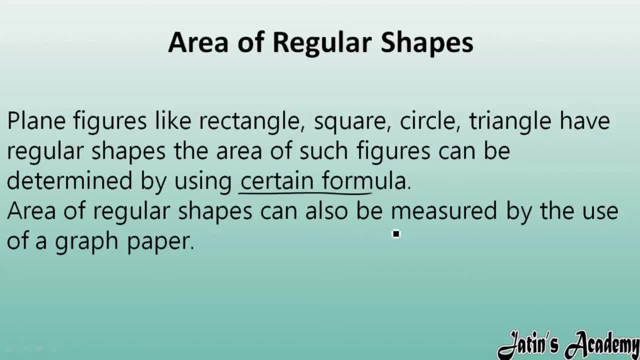 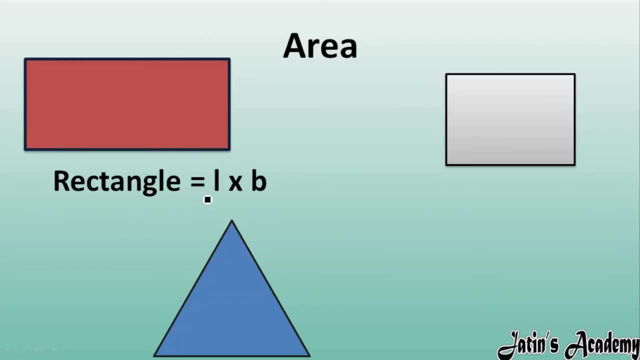 Even though area of regular shape can also be measured. We can use, even though, a graph in order to measure the area of regular shape. Fine, So here we are having different area, like first, we are having rectangle. This is a form, plain figure of rectangle. 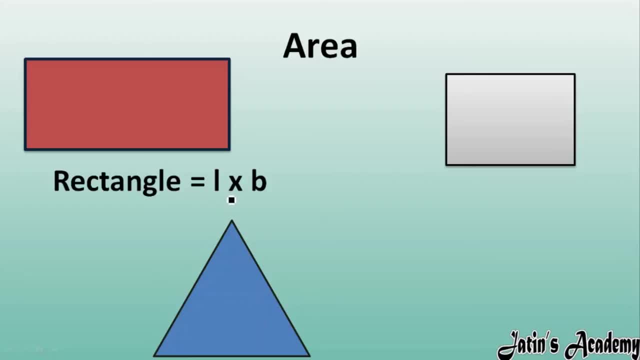 So how to find the area of rectangle? by using the appropriate formula, that is, length multiply breadth. Here, for example, this is a length of rectangle and this is breadth of rectangle, by knowing its length and breadth, which we are going to study, or we are going to calculate its area. 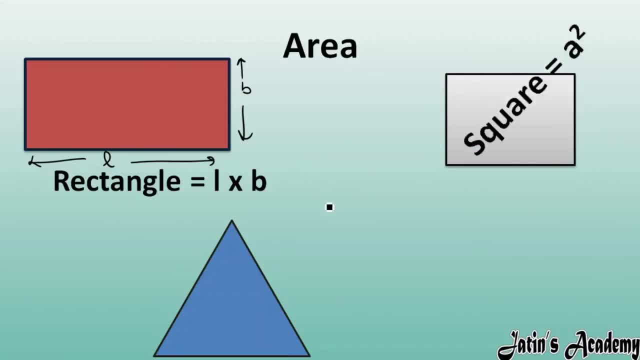 We are going to study or we are going to calculate its area. We are going to study or we are going to calculate its area. Second, we are having square. So how we can find the area of square? by multiplying the sides. For example, this is a side A. 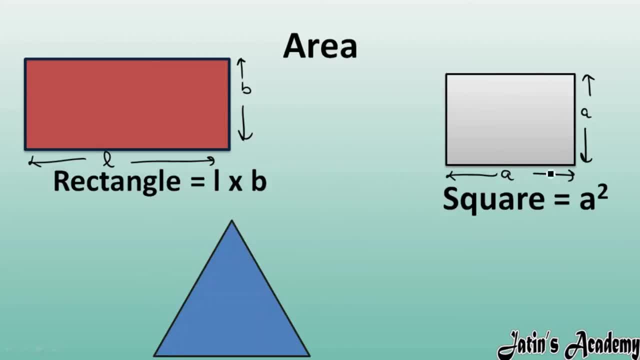 Similarly, this is also A side. Why? Because in area in square, all sides are equal. If this is A side, this is also A side. So what is the area of square Side, multiply side? that is A multiply A, A square. 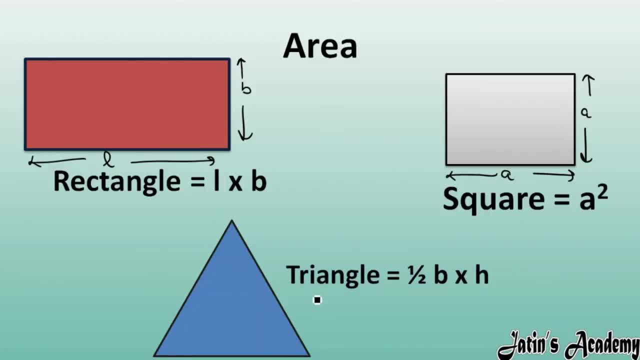 Fine. Next we are having triangle. So how to find the area of triangle? by using the formula one by two, base multiply height. This is the base of triangle and this is the height of triangle. by knowing the base and height, we can simply measure. 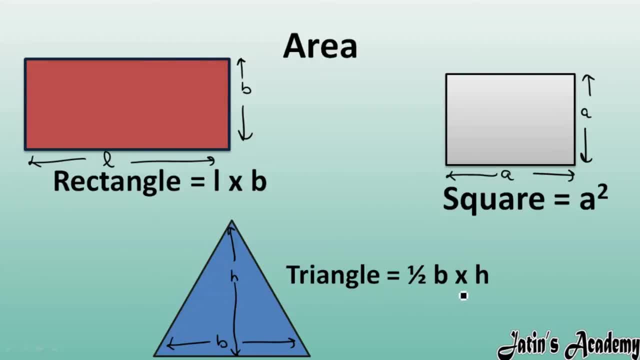 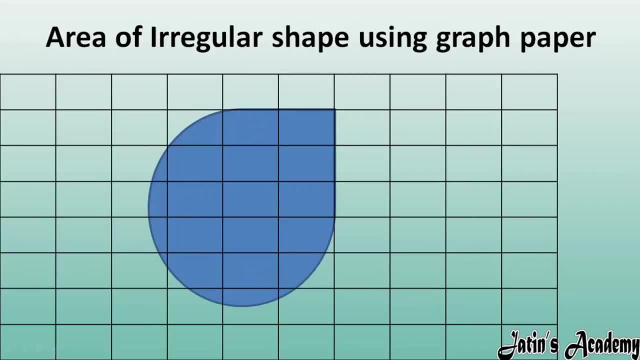 We can simply use the formula that is, one by two base multiply height, in order to know the area of triangle. Next, we have area of irregular shape using graph paper, as we have learnt now only that for the regular shape we are having some kind of appropriate formulas for by using the appropriate formulas, 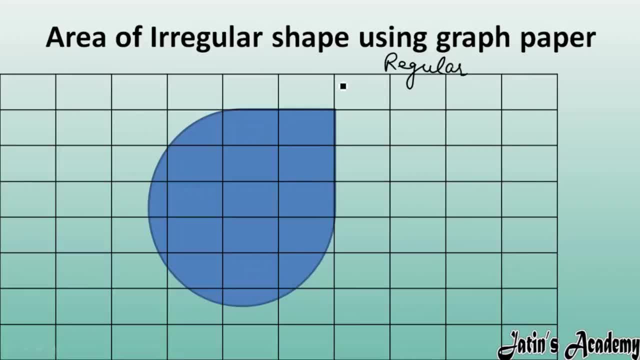 You can use that formulas and you can find the area of regular shapes. But now is the problem for irregular shaped object. If I am having this kind of irregular shape object, so I am not having any kind of formula in order to know the area of this irregular shaped object. 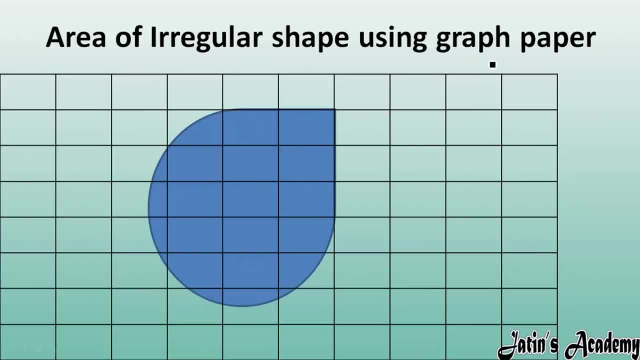 So now, what is the method to calculate the area of irregular shape? The method is by using a graph paper. For example, this is a graph paper and this grid, This one box, is of one centimeter square area. Here also One centimeter length. breadth, also one centimeter. 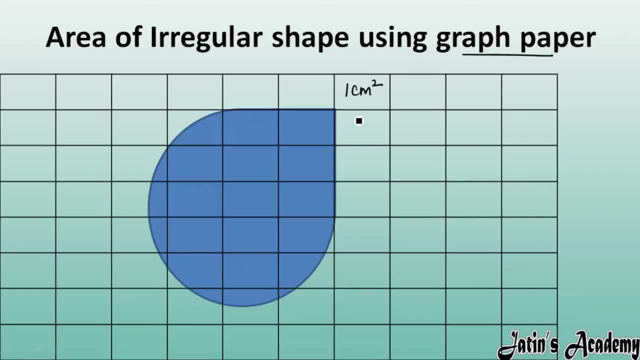 So area will be length multiply breadth, that is one centimeter square. find, For example, this area of one grid is one centimeter square. Now we have to find the area of the sleeve. So what we can do, Firstly, you can write the area. 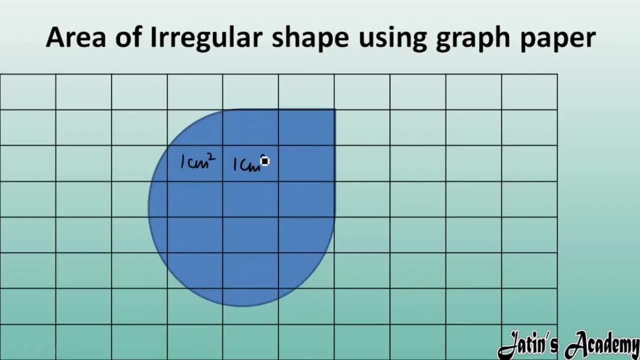 For example, this box is having one centimeter square. This also one centimeter square. Just write all the one centimeter squares to that box, which is fully filled by the leaf. So these areas are fully filled by the leaf. So these areas are fully filled by the leaf. 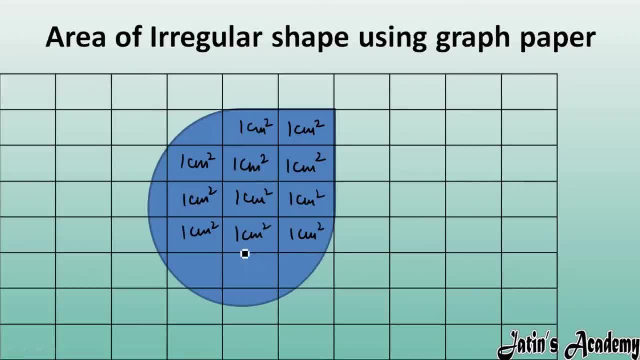 So just write one centimeter square here, Okay, And this is also approximately fully filled, Approximately fully filled. You can also write one centimeter square, But you can check these one Here. you can see this area is half filled only. 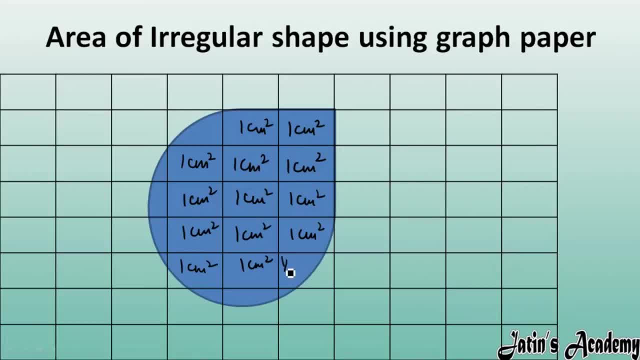 In this one grid. this area is half filled only So you can write here half centimeter square. This also total. I am going to take here this one from here to this. This is also half filled, So half centimeter square. 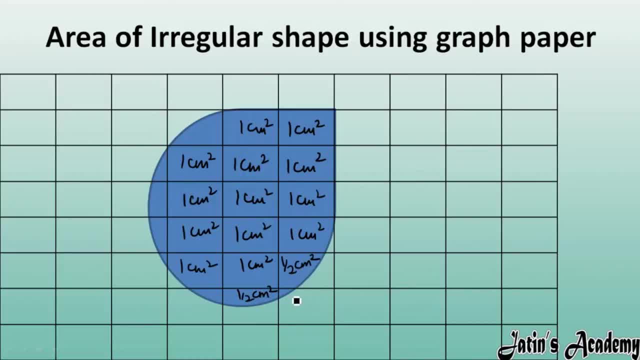 This is very small area You can neglect This is also very small area You can neglect, No problem. This you can take half centimeter square Here. this also, this total, I can take half because it is less than half. This is also less than half. 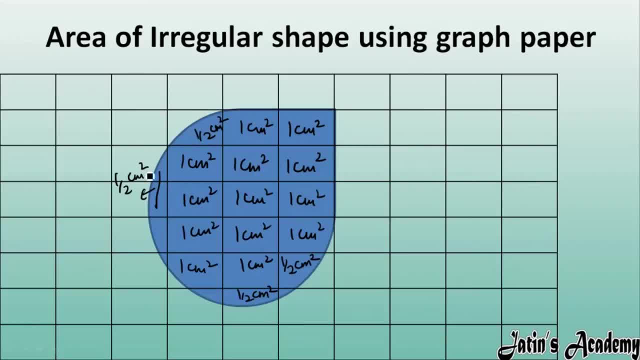 So this total, I am going to take half centimeter square And this also total, I am going to take half centimeter square. So, after writing these all things, what you can do, You can just plus add up all these centimeter square. 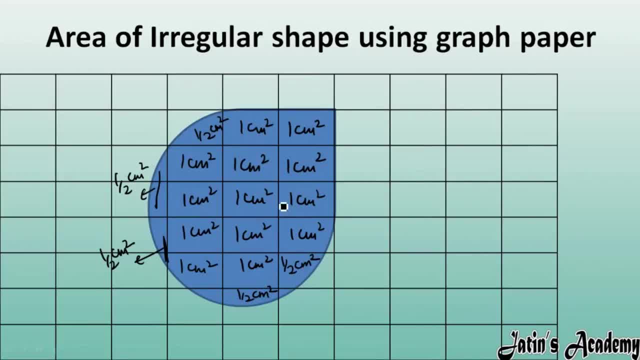 So how we can plus One, two, three, four, five, six, Seven, eight, nine, ten, eleven, twelve, thirteen, Thirteen centimeter square is full one. Now check the half ones: One, two, half and half means one. 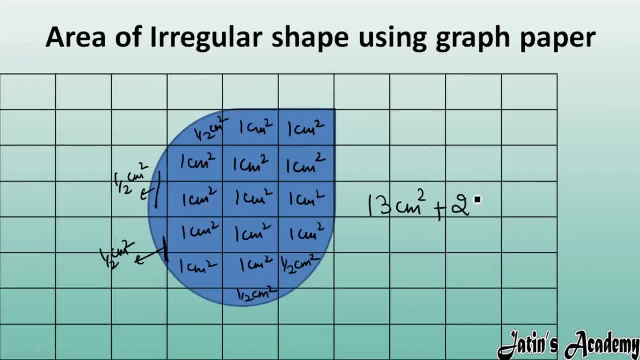 This half and half means two, And this half means two and half. So here it is two and half centimeter square. So what will be the answer? Thirteen plus two, Fifteen and half centimeter square is the area of this irregular shaped object. 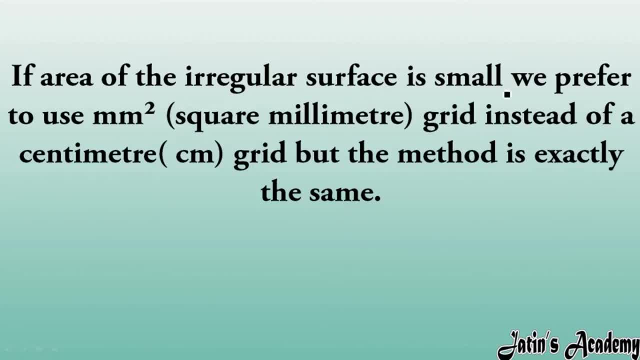 If the area, If the area of irregular surface is very small. If area of irregular surface is very small means, for example, this much only area we are having for irregular surface. We prefer to use millimeter square grid, So this grid which we are using of a graph paper instead of one centimeter. 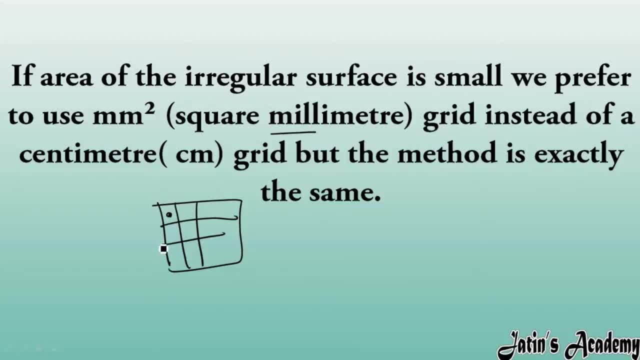 we can also use of one millimeter square. Okay, Instead of using centimeter, we are using here millimeter for the very small irregular surface. Fine, But the formula which we are using means to count the box. That formula is going to the same. 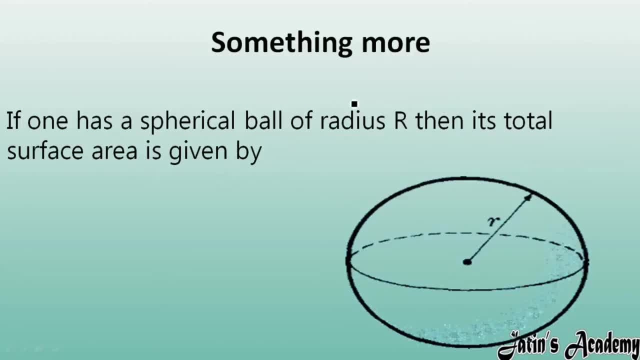 Method is exactly the same. Next, we are having something more to you, Something more for you. I want to tell you, If one has a spherical ball of radius r, If I am having this spherical ball of radius r, Then its total surface area, 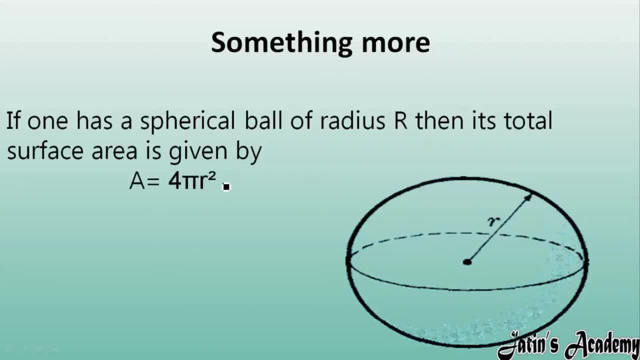 Total surface area of this sphere is given by 4 pi r square, If someone ask you about the total surface area of sphere. So total surface area of this sphere is given by 4 pi r square. So total surface area of sphere is what. 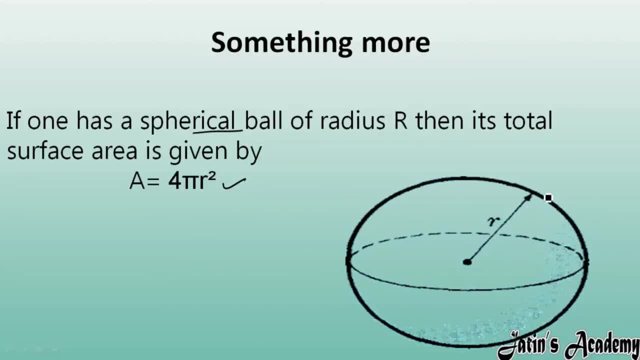 4 pi r square, where r is the radius of this square. Pi is a constant value, 22 by 7, or you can write 3.14.. This is always a constant value. Same value we have to put in all the formulas. 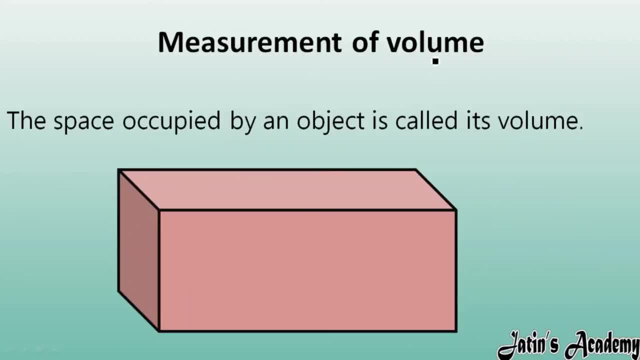 Fine. Next we are having measurement of volume. Till this we are having the measurement of area. Now we are going to start the measurement of volume. So first of all, we should know what is volume. Volume is the space occupied by an object. 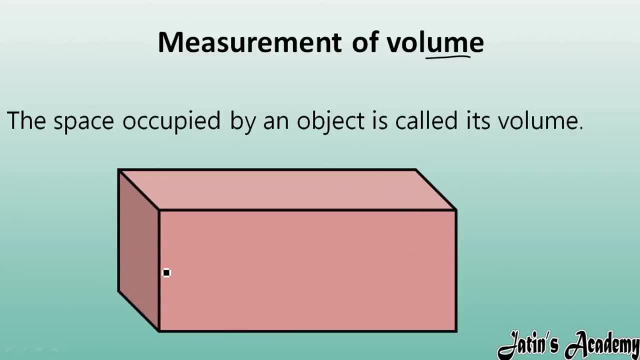 For example this object I am having. So the space occupied means length, breadth and height. Occupied 3 dimensional space occupied by this object is nothing but its volume. Fine, Next we are having SI unit of volume. So SI unit of volume is meter cube. 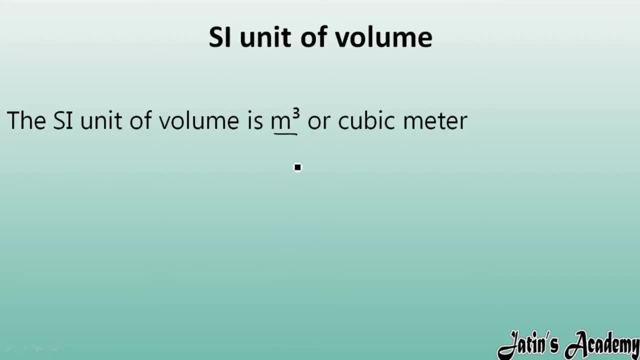 Why we are having meter cube, not why we are not having here meter square, Because in area we are having just length and breadth of any plane In figure, but in volume we are having length also, we are having breadth also, even though we are having height also. 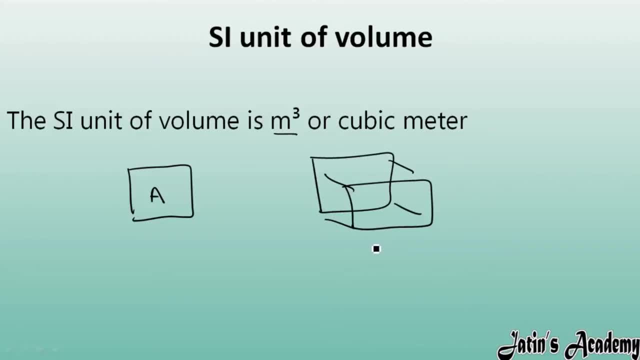 So 3 measurements are there, 3 physical quantities are there. length is also there, breadth is also there, height is also there. That is why here we are using meter cube. So SI unit of volume is meter cube and CGS unit of volume is centimeter cube. 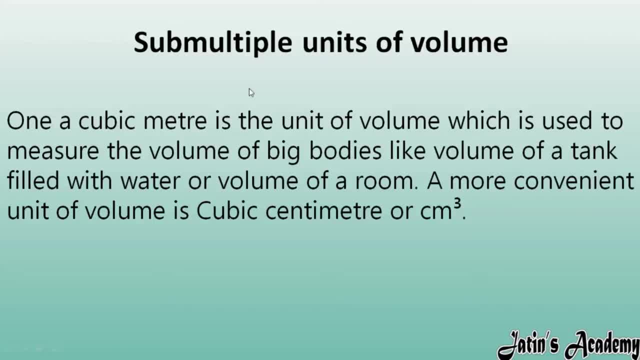 Next we are having sub-multiples units of volume. So now we are going to study about the sub-multiples units of volume. So now we are going to study about the sub-multiples as well, as here only we will study about the multiples, also of volume. 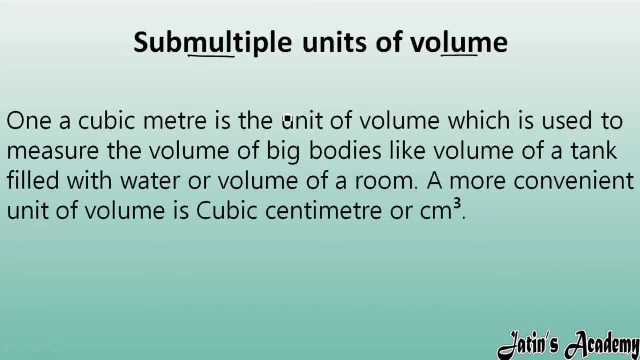 So what do you mean by sub-multiples and multiple Sub-multiple units? are that units which are used for smaller measurement, If I am having very small volume. So for very small volume, which physical quantity I am using here or which unit I am going to use here? 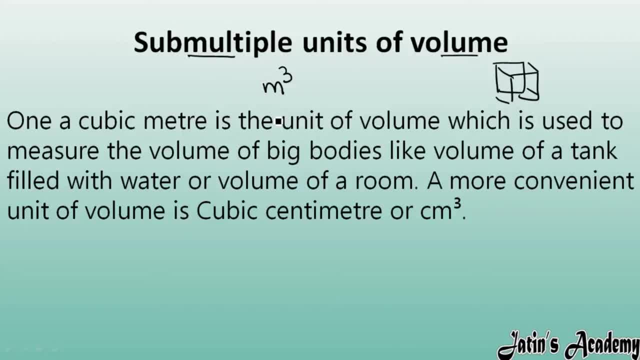 So, as we know, meter cube. meter cube is a unit of volume which we are using for the volume of big bodies. Meter cube is SI unit which we are using for the big bodies. So meter cube is SI unit which we are using for the volume of big bodies, like volume of tank filled with water, okay, or volume of room. 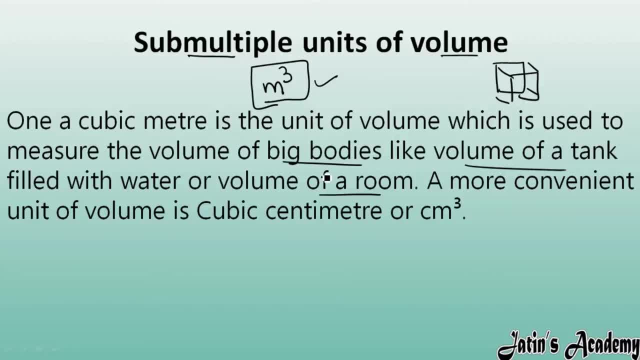 So meter cube you can use for, like bigger bodies, But if I am going to use for the smaller body, So if I am having very small like object and I want to measure the volume of this very small object, So which units I am going to use here for the smaller measurement I am going to use centimeter cube. 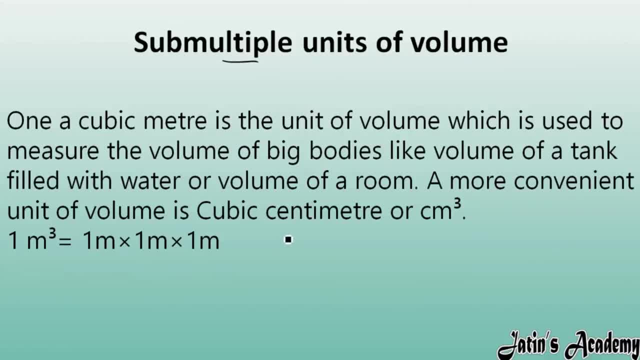 So here we are having relation: 1 meter cube, So 1 meter cube. we are going to write it as 1 meter multiply 1 meter multiply 1 meter, So as 1 meter is equals to 100 centimeter. 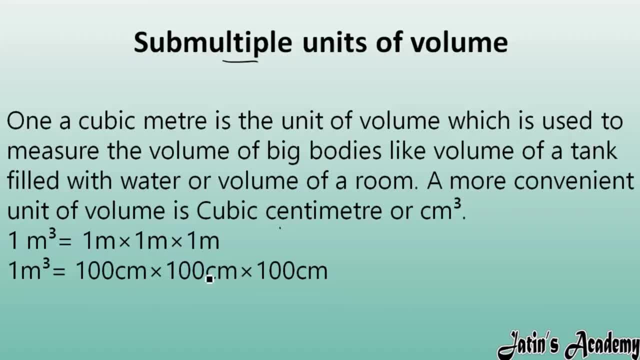 So instead of 1 meter we are going to write 100 centimeter, 100 centimeter, 100 centimeter. So 1 meter cube is equals to this much centimeter cube. This is the relation between SI unit and CGS unit of volume. 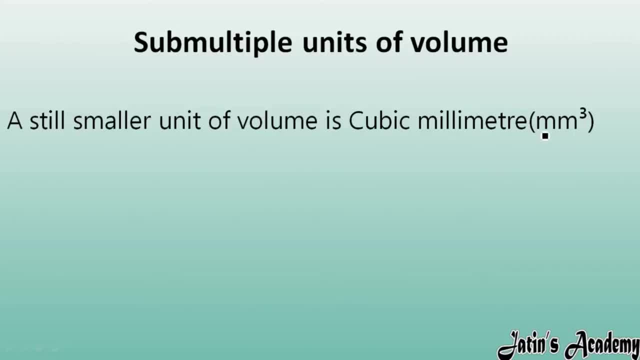 A still smaller unit for the volume is mm cube. Centimeter cube is also smaller unit or sub multiple of volume, if you want to see any smaller unit of volume. so that is millimeter cube. millimeter cube is also the sum multiple of the measurement of volume. so here we. 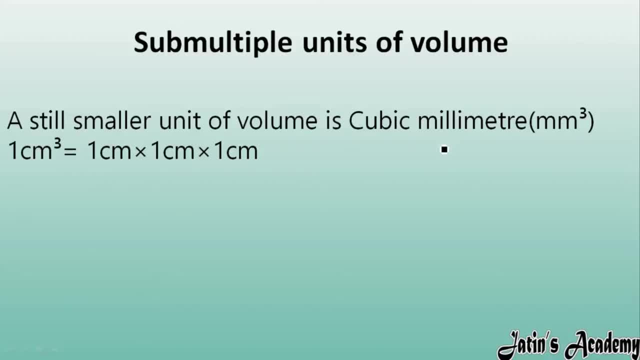 are going to write the relationship between 1 centimeter cube and 1 millimeter cube. so 1 centimeter cube can we write it as 1 centimeter multiply 1 centimeter multiply 1 centimeter and we know 1 centimeter is equals to 10. 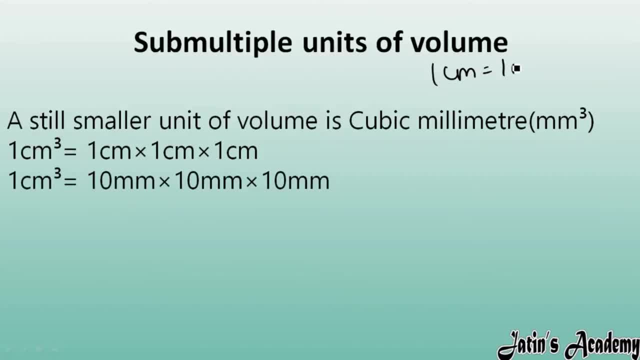 millimeter. 1 centimeter is always equals to 10 millimeter instead of 1 centimeter. I am going to write here 10 millimeter, 10 millimeter and 10 millimeter, so by solving it we can get 1 centimeter. cube is equals to 1000 meter. 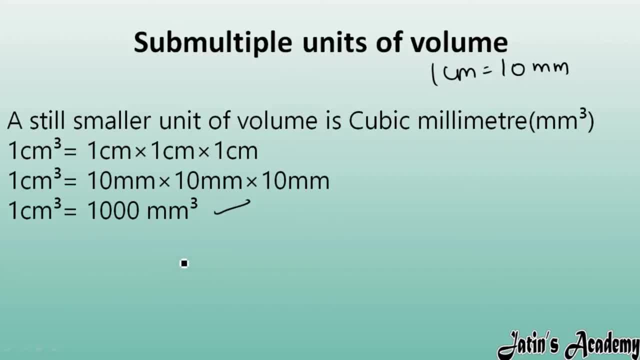 cube. this is very important relation from paper, exam or paper or exam point of view that 1 centimeter cube, like this question will ask to you: 1 centimeter cube is equals to dash millimeter cube. so here you have. 10 millimeter cube equals to 10 millimeter cube. so here you have. 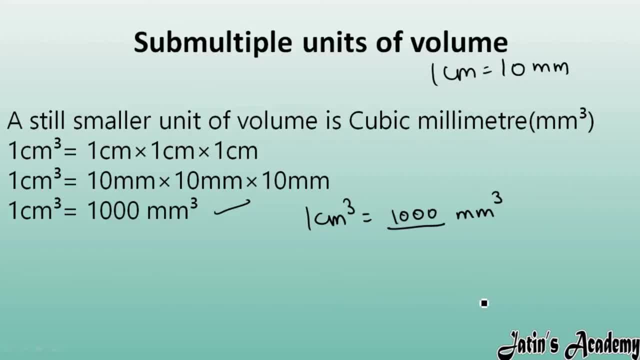 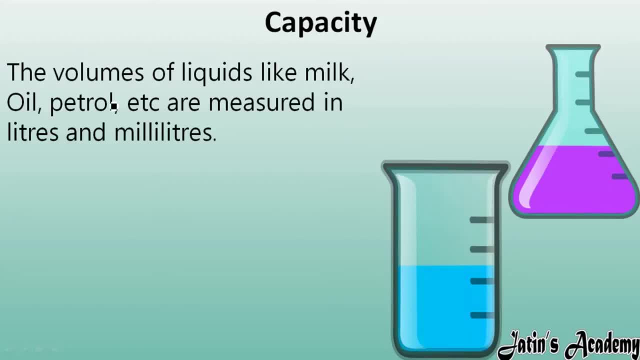 to put the value thousand millimeter cube. next topic: we are having capacity. so what do you mean by capacity? the volume of liquid like milk oil, petrol, etc. are measured in liters and milliliter, as we know whenever we are going to some shop in order to like buy some oil, petrol. so there we are. 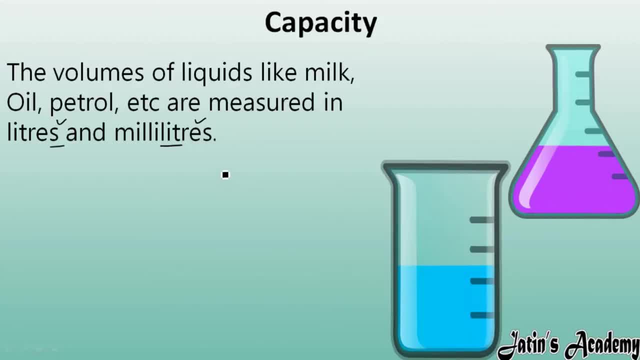 using the terms liter and milliliter in order to measure the volume of that liquids. so we should know what is capacity? capacity means the inner volume of the container which holds a liquid. so this inner volume of this container which this can hold a liquid, that is known as its capacity. 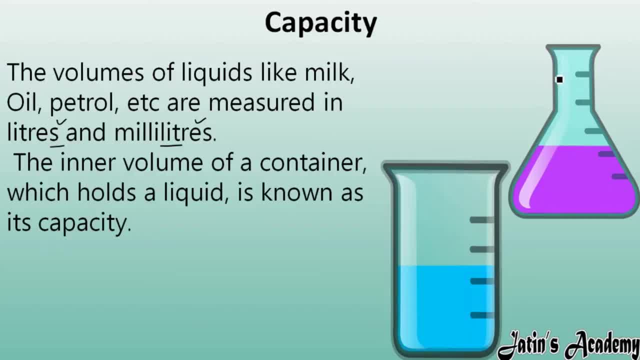 so what is the capacity of this like glass? what is the capacity of this conical flask? capacity means the amount of volume or the inner volume of the container which holds a liquid. that much amount of that much volume of the container is known as its capacity. next we are: 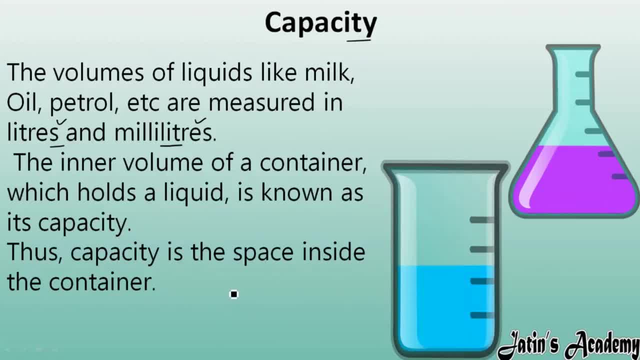 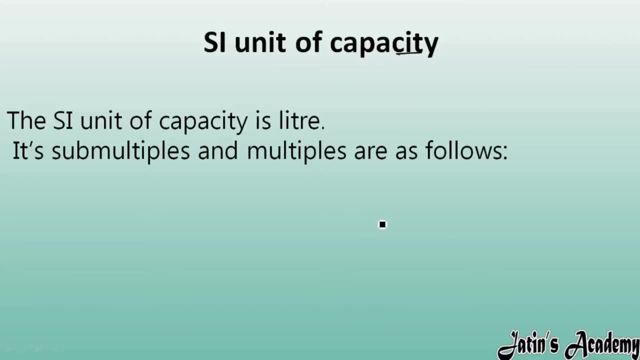 having capacity is the space inside the container. or you can write like this also: that capacity is the space. whatever space is present inside this container which can hold a liquid, that space is nothing but its capacity. next, we are having si unit of capacity. as we know whenever we are using 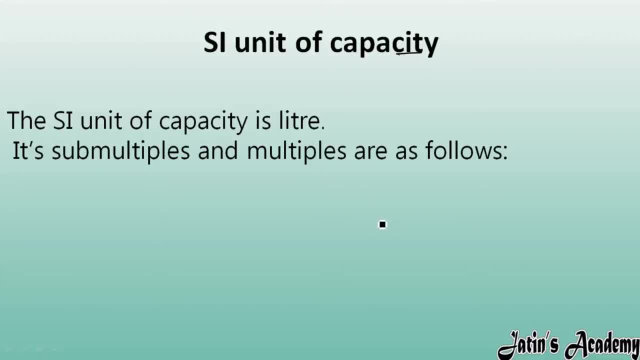 any physical quantity, that time we are using its some units and even though we are using some si units, since system international the units. so the si unit system of capacity is liter. si unit is liter and its sub multiples and multiples are also there like other physical quantities. 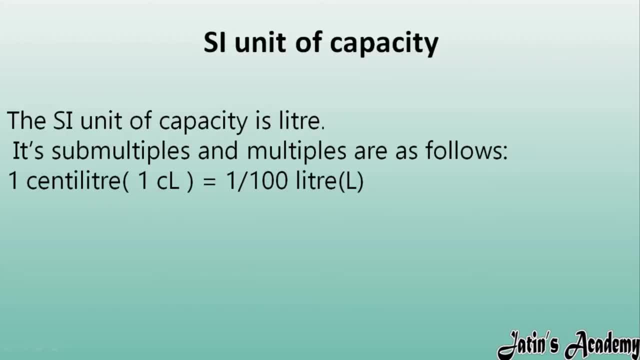 so sub multiple is centiliter. 1 centiliter is equals to 1 by 100 liter, and when we are having milliliter, 1 milliliter is equals to 1 by 10 centiliter, or you can say 1 by 1000 liter, as. 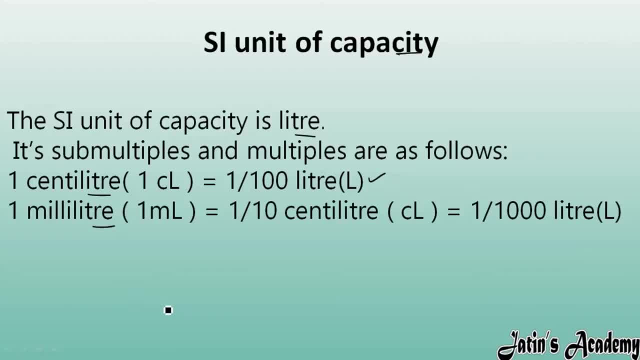 later is its si unit. so Centilitre and millilitre are its sub-multiples. Next we are having its multiple. This is its multiple kilolitre. So 1 kilolitre is equals to 1000 litres. And next we are having volume of regular solids. 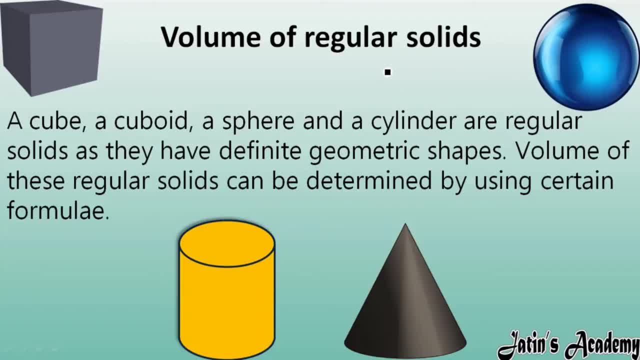 So how to measure the volume of regular solids and what are regular solids? Now we are going to study that A cube, cuboid sphere and a cylinder are regular solids, Means whatever things we are watching in our surrounding that are having fixed like length. 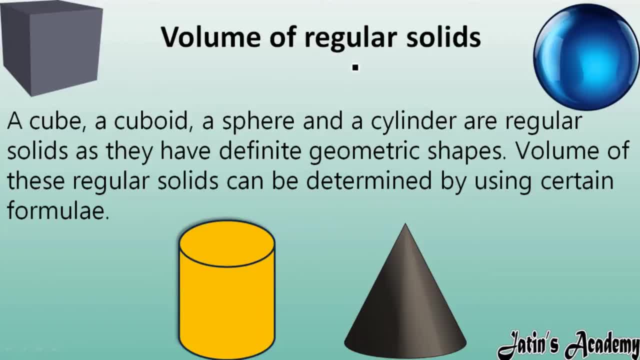 fixed height or fixed diameter radius, that all solids are known as regular solids, For example, cube, cuboid, sphere, cylinder. They all are regular solid as they have definite geometric shape. because they are having all definite geometric shape and volume of these regular solids can be determined by using certain formulas. 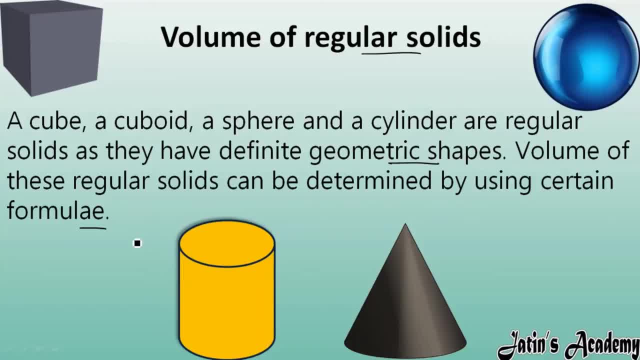 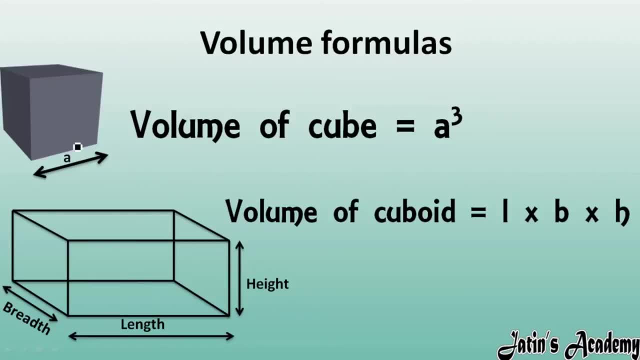 And what are that formulas? In the next slide we are going to study about the formulas of regular solids. So here we are having formulas for the volume. First we are having volume of cube. This is a cube And, for example, the side or the edge of this cube is A. 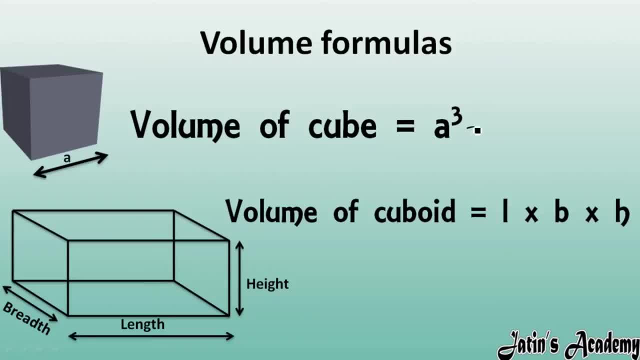 So what is its volume? Volume of cube is side cube. That is A multiply A. multiply A means three times. we have to multiply the side, We will get the volume. Next we are having volume of cuboid. This is a kind of cuboid which is having some kind of length, which is having breadth and height. 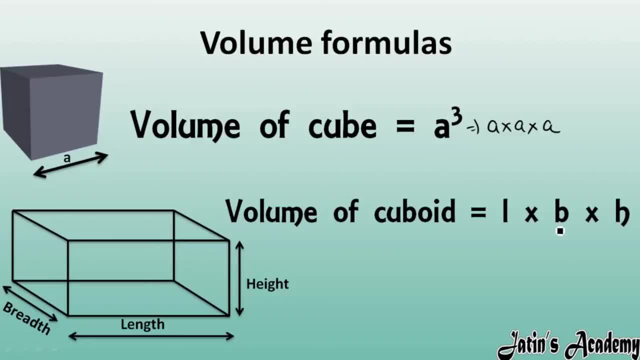 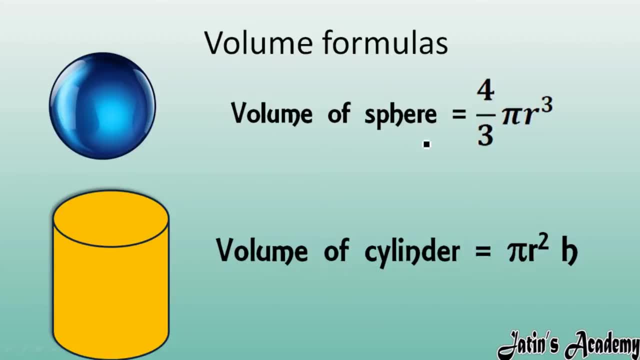 So how to measure the volume of cuboid? by using the formula length multiply breadth, multiply height. Next we are having volume of sphere. This is a kind of sphere. So how to measure the volume of sphere? by using the formula four by three, pi r cube. 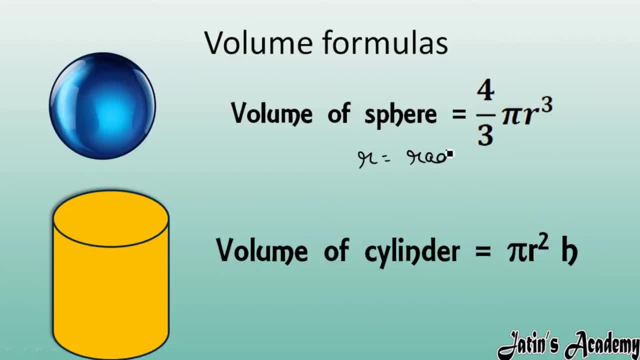 So what do you mean by here? r means radius of sphere, r means this one radius of sphere. And what do you mean by pi? Pi is a constant value. that is twenty two by seven. In all numericals we are going to use the same pi value, that is twenty two by seven. or you can use three point one, four also. this is also same value. fine, four by three is constant. pi is constant by knowing its radius. 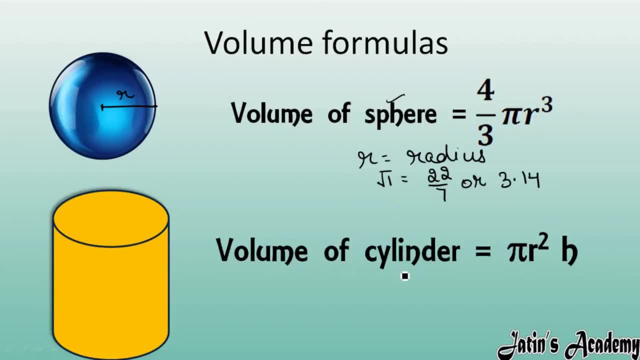 We will calculate the volume of sphere. Next we are having volume of cylinder. This is a kind of cylinder. So here in cylinder, this is a radius of cylinder, This is the height of cylinder. fine, So by using the formula pi r square h, where pi is some constant value. 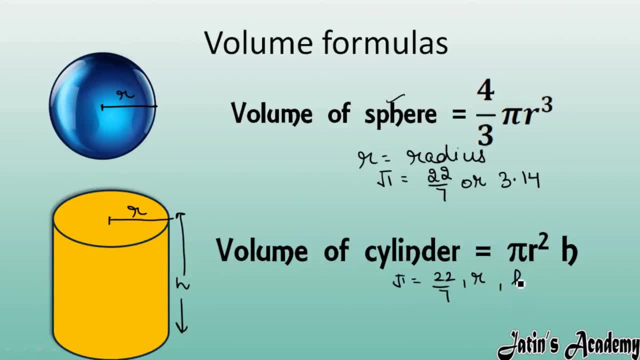 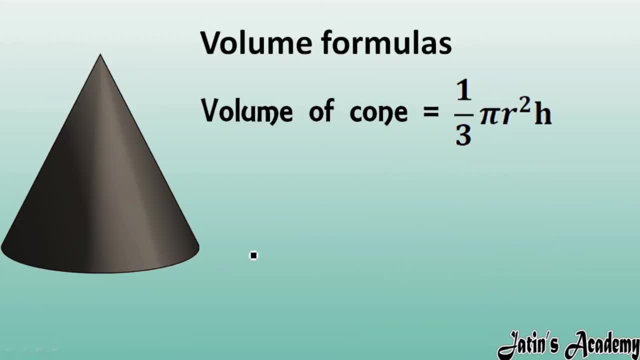 Twenty Two by seven. r is the radius of cylinder and h means this height of cylinder. By knowing all these values, we will calculate the volume of cylinder. Next, we are having volume of cone. So how to measure the volume of cone? 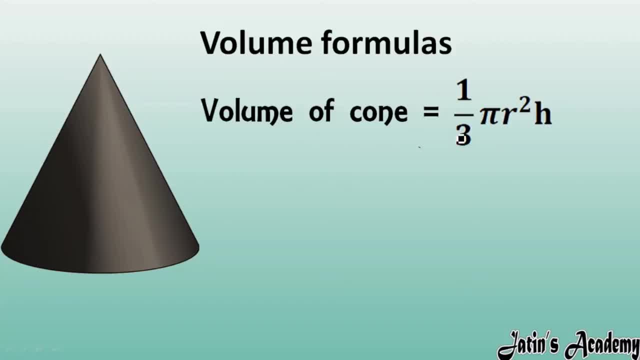 First of all, this is a kind of cone. Okay, so how to measure the volume of cone? by using formula one, by three pi r square h. So here, what do you mean by r? r is a radius. r is a radius of this cone, h means the height of. 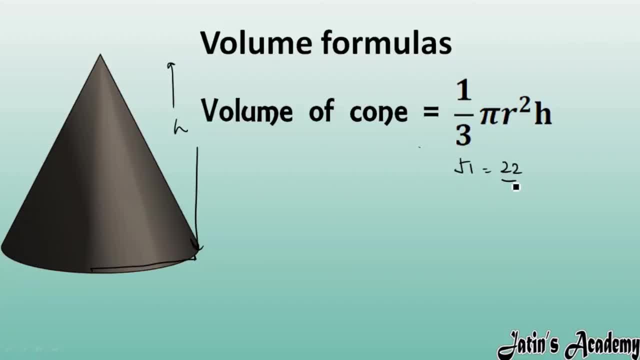 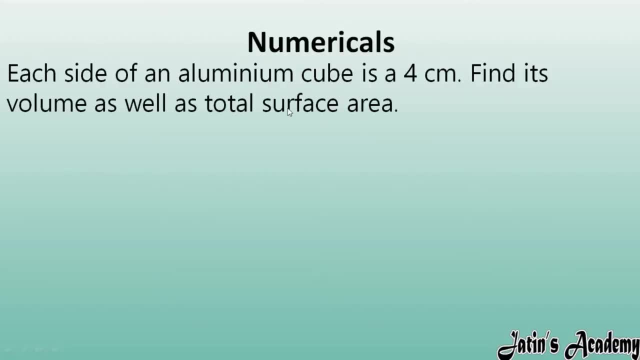 this cone and pi value now might be, you are knowing that is twenty two by seven, that is constant value. Next we are having numericals related to this. So first we are having: each side of an aluminium cube is a four centimetre. 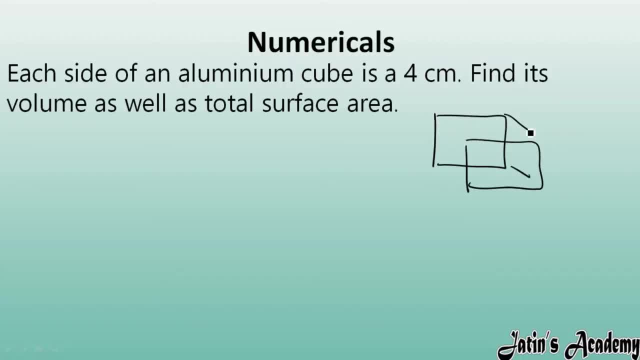 So here I'm having one aluminium cube and the side of aluminium cube is four centimetre. Find its volume as well as total surface area. So here I'm going to find the volume as well as total surface area Of this cube. So now only we have studied about the volume of cube. 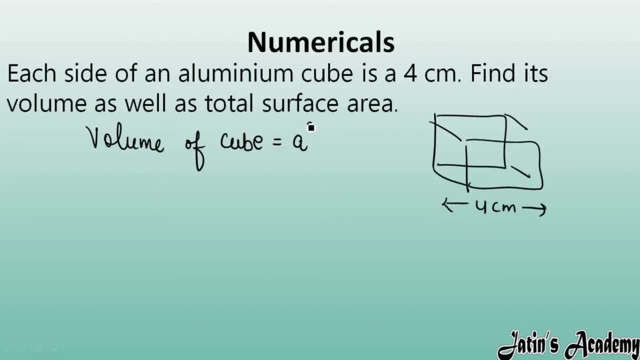 So what? what is the volume of cube? volume of cube is side cube, So side value. we have given that is four cube. here I'm going to put the value. So four means what? four? the power cube means four, multiply four. multiply four means four. 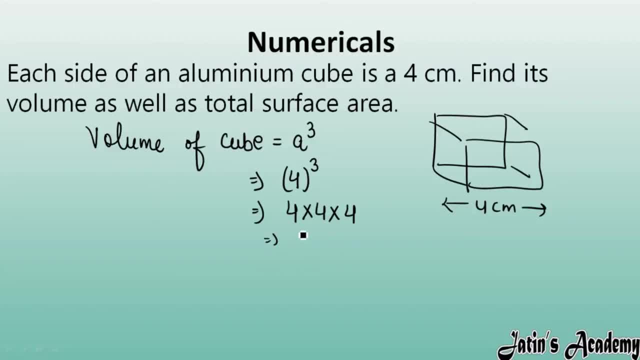 We have to multiply three times. So here answer will be sixty four centimetre cube, fine. Next we have to find the total surface area. This formula We have to remember: total surface area of cube. So total surface area of cube is six side square. 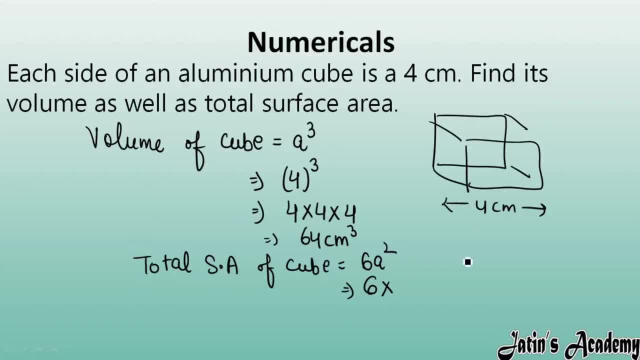 So six side square means six multiply side square side square is four square. So here you can solve six multiply four, multiply four. by solving what you will get, You will get ninety six centimetre square. Why here I'm using centimetre cube and why here I'm using centimetre square? 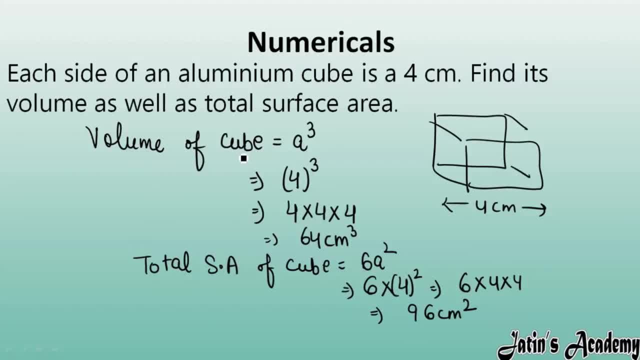 Listen carefully. here Actually I'm calculating The volume of cube and cube. You can see here cube is volume is always in a centimetre, cube always in a cubic metre- Okay, or cubic centimetre, But here surface area is always in centimetre square or metre square. 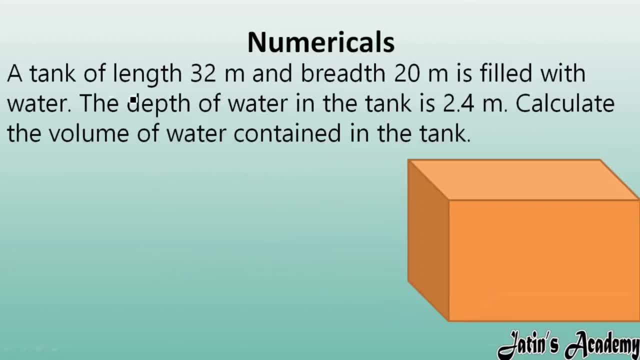 According to the units next numerical, We are having a tank of length 32 metre and breadth 20 metre. is filled with water, For example, this kind of tank we are having, which is having length. So here length of tank is given, Length of tank is equals to 32 metre and its breadth is also given. 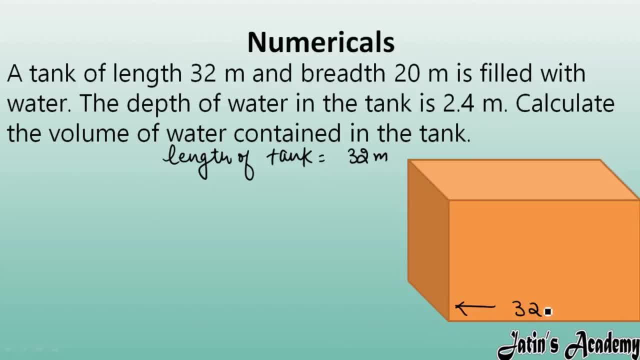 For example, this is length of tank. This is length of tank: 32 metre and this is breadth of tank. breadth is 20 metre. fine, So breadth of tank is equals to 20 metre. is filled with water. This tank we have to fill with water. 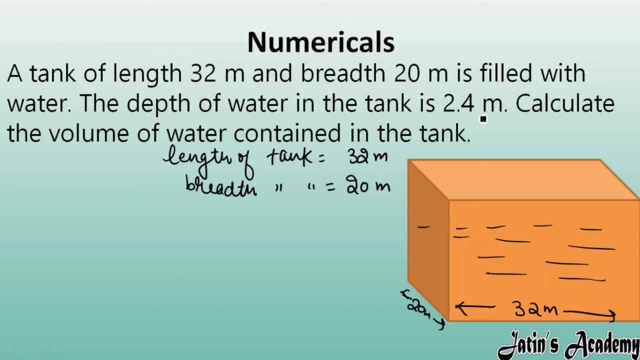 So it is filled with water. The depth of the water tank is 2.4.. This depth Water is 2.4 metre. We have to calculate the volume of water contained. this volume of water contained in this tank, We have to calculate. 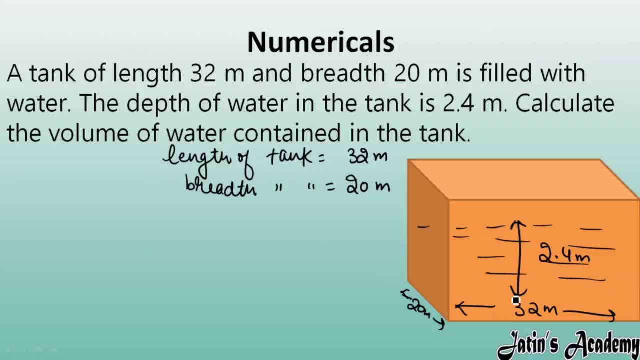 So here you can see, this is given length, breadth and this is given height. So easily we can measure the volume. So what is the volume of cuboid? volume of cuboid is nothing but length, multiply breadth, multiply height. So just put the values: length is 32 metre multiply. 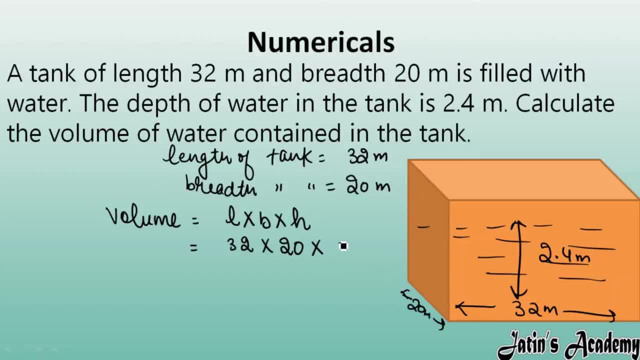 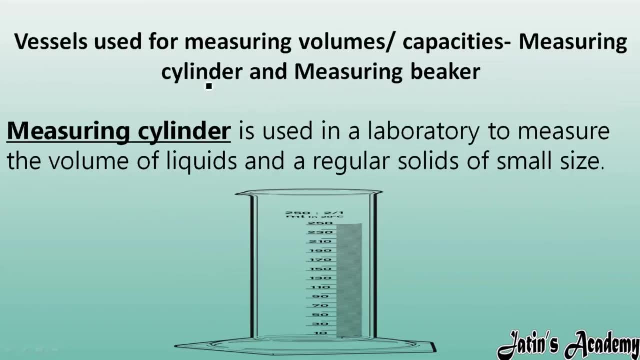 Breadth is 20 metre. multiply Height is what 2.4. Meter. So by multiplication, by solving what, you will get 1536 metre cube as the answer of volume contained in this tank. Next, we are having vessels used for measuring volumes. 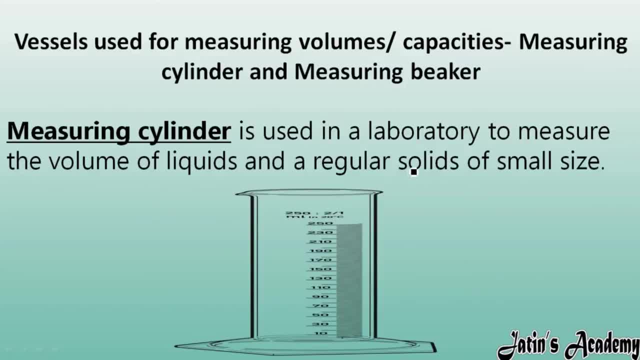 So now, which vessels we are going to use in the like chemistry lab or physics lab in order to know or in order to means measure the volumes or capacity. So here we are having some of the vessels. first We are having measuring cylinder. Measuring cylinder is usually used in laboratories in order to measure the volume of liquids and even though we can measure the regular solids also, volume of regular solid, also of small size, by using this measuring cylinder, fine. next vessel: 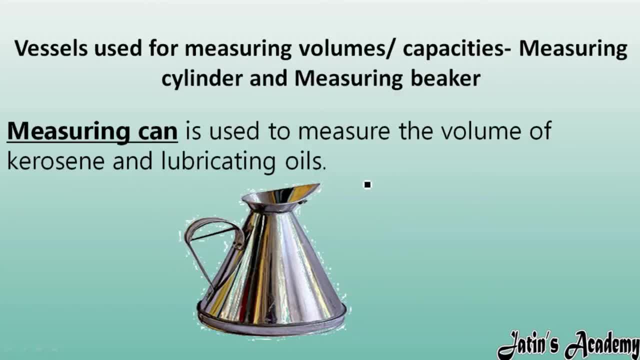 We are having measuring can. this is a form of measuring can in which we are going to measure the volume of kerosene or lubricating oils. If you want to measure the volume of kerosene or lubricant oils, then we are using the measuring can. 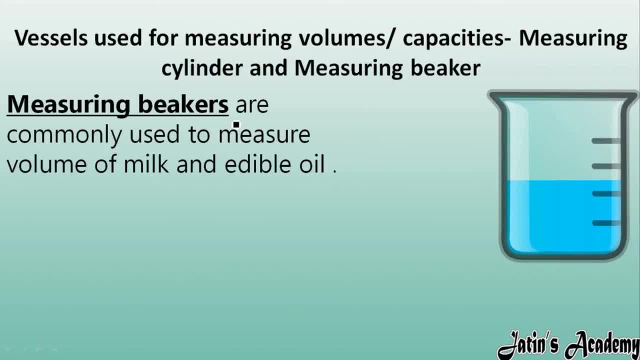 Next, we are having vessels used. that is, third, measuring beaker. So measuring beaker is commonly used in order to measure the volume of milk, or used to measure the volume of edible oil. This is a form of measuring beaker. This is also we are using in chemistry or physics lab also fine, 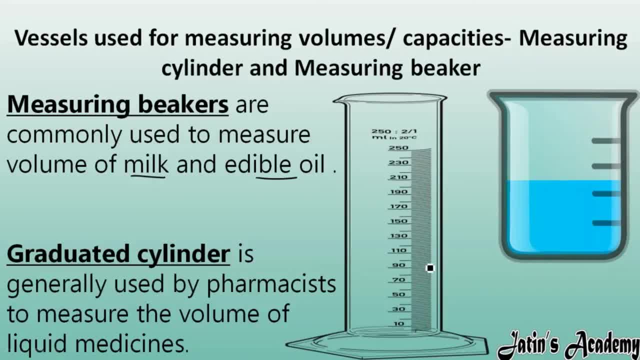 Next we are having graduated slender. Why this name is graduated? because here some marks are given, some graduations are given, So it is generally used by pharmacist. So pharmacist They are using in order to measure the volume of Liquid medicines, if they are giving liquid medicines to any patient. 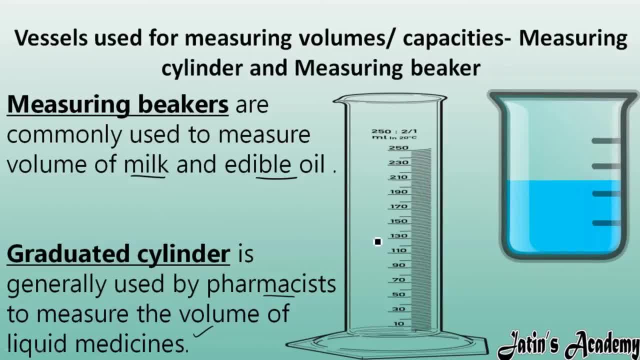 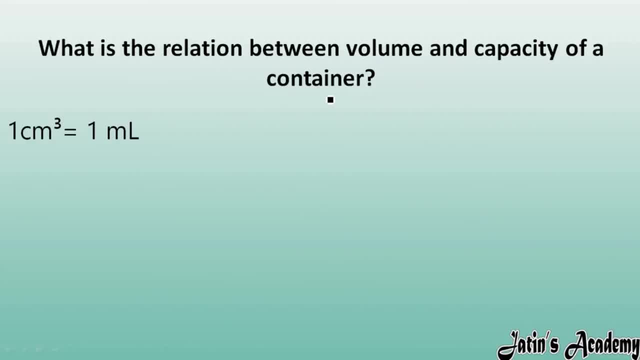 So in order to measure the volume of that liquid medicine, they are using this graduated slender. Next we are having: what is the relationship between volume and capacity of a container? So now we are going to see the relation between volume and capacity. as we know, volume is a three-dimensional space occupied by an object, and capacity is the inner volume of any container. fine, 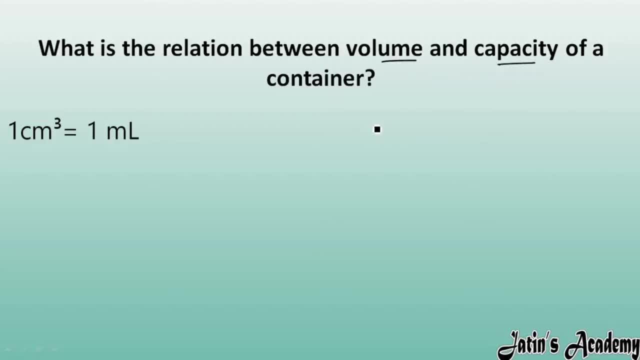 So now we are going to do the relation between the Volume and capacity of container. So volume, we know it is centimeter cube. capacity, We know milliliter. This is first relations, a relationship: one centimeter cube is equals to one milliliter. 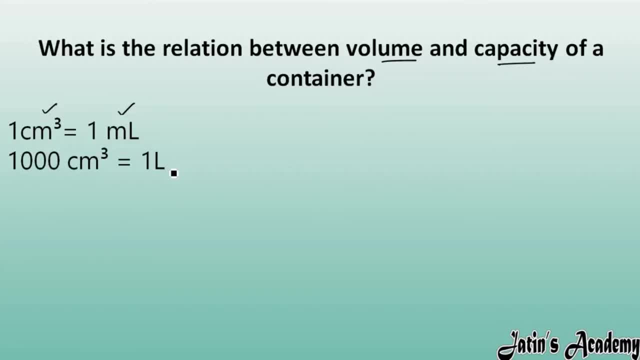 Next we are having: thousand centimeter cube is equals to one liter. This is very important from exam points of view. also, that one centimeter cube is equals to dash milliliter. or they can ask: thousand centimeter cube is equals to dash liter. So here you need to put: 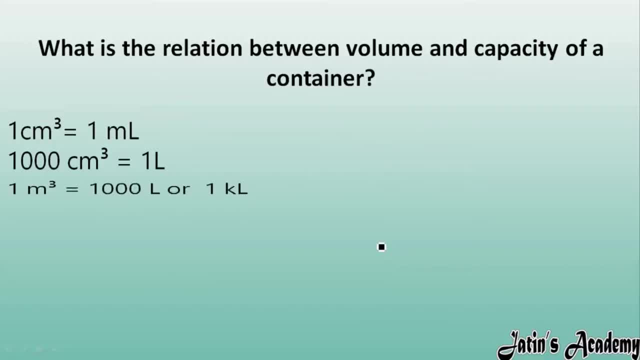 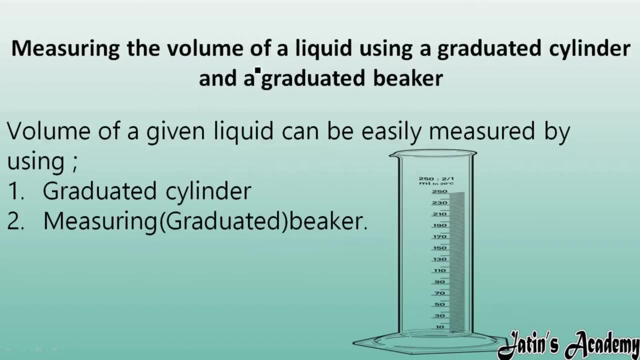 The values one and one, fine. Next, we are having one meter cube. one meter cube is equals to thousand liter, or you can say one kiloliter. This relation is also very important. Next, we are having measuring the volume of a liquid using graduated slender and graduated beaker. 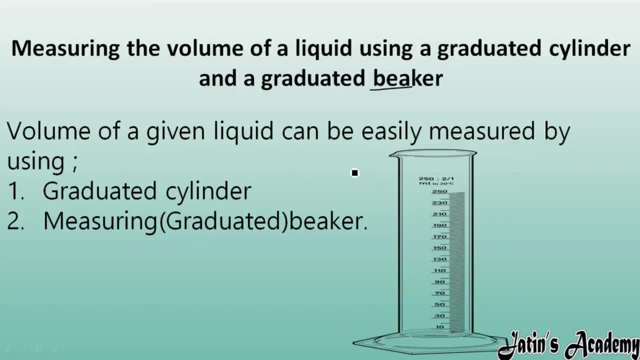 Now we have started that many vessels are there in order to measure the volume. Now, how to use that- measuring slender or graduated Beaker, graduated slender- how to use them. Now we are going to study one by one. So the volume of given liquid can be easily measured by using graduated slender and by using graduated beaker. 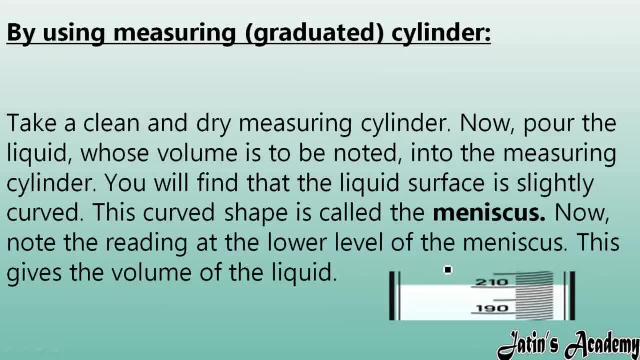 So let us see, by using measuring slender, how to like find the volume of any liquid by using graduated slender. First of all, we have to take the clean and dry measuring slender. Now we have to pour the liquid. for example, in this beaker, one liquid is there and I have to check the volume of. 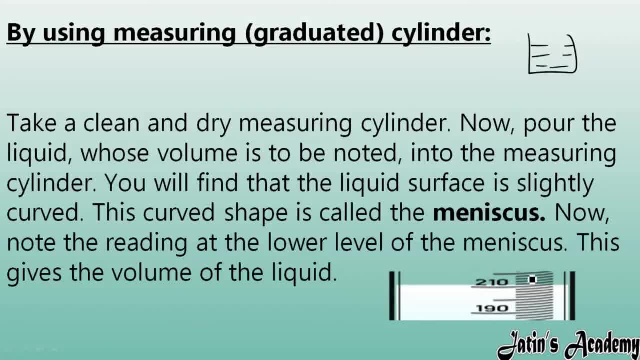 This liquid. fine. So what I will do? I will take one like dry and clean measuring slender. Now I will pour this volume, this liquid. I will pour into this measuring slender Now I will find that some kind of liquid surface is there here. one curved surface is formed in the measuring slender. 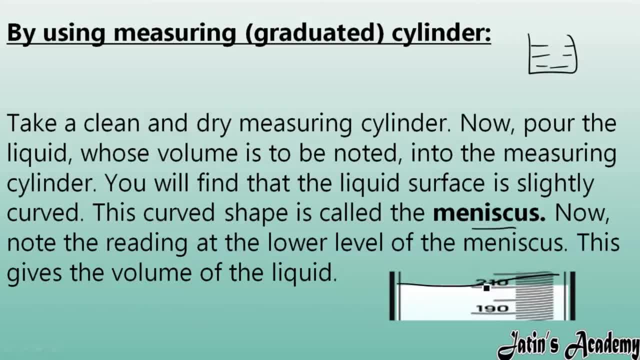 So this curved surface is curved Shape is nothing but a meniscus. meniscus means what? the curved surface which is formed at the upper layer of liquid. that is a meniscus. Now we have to note The reading of this meniscus. as you can see here, reading is 210.. 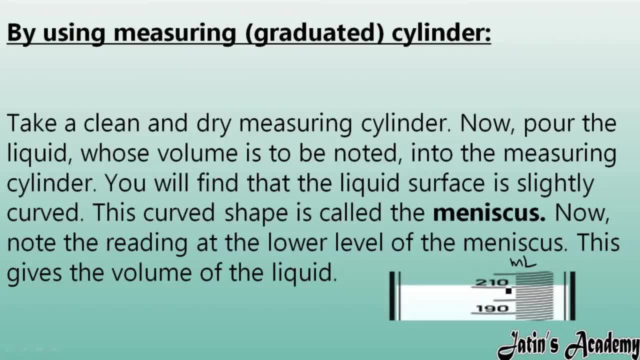 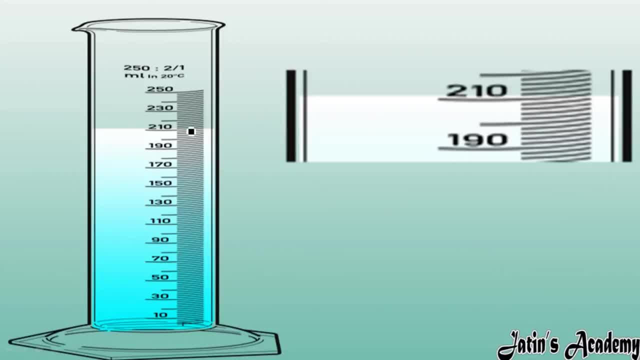 So where this volume of liquid must be 210, if it is in ml, then 210 ml, fine. So this is a way you can say full-fledged measuring. slender here. This much volume, this much meniscus is there. here You can note down the reading. 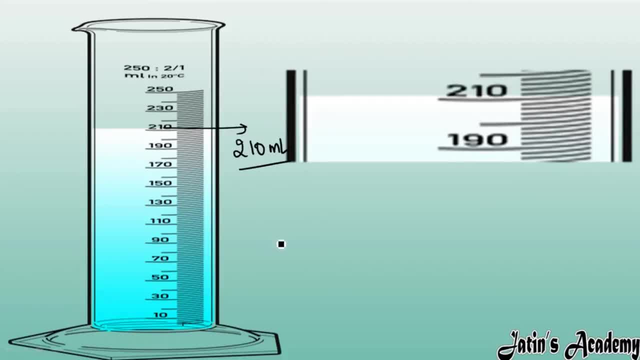 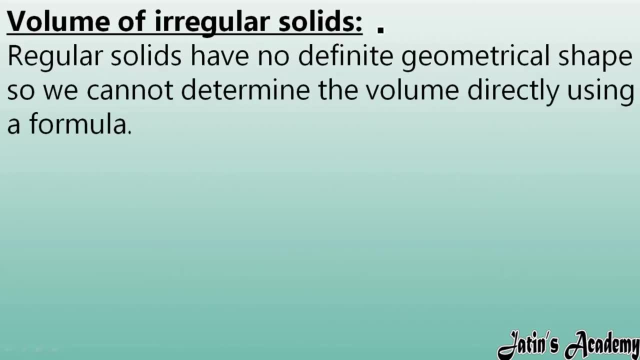 So here, volume of liquid is 210 ml. So by this way, simply, we can measure the volume of any liquid, fine. Next, we are having volume of Irregular solids. now how to measure the volume of irregular solids? that we have to study first of all. 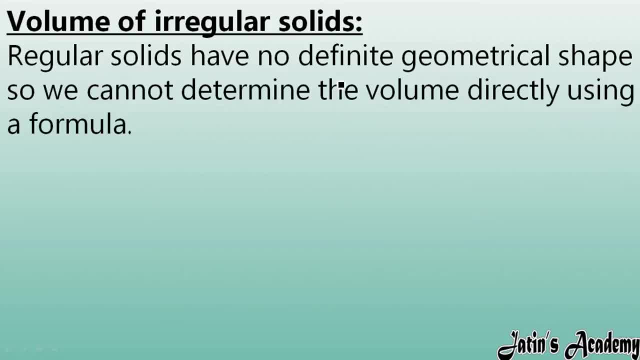 What are irregular solids? irregular solids are that solids which do not have any definite geometrical shape. Okay, and we cannot determine the volume of that irregular shape object directly by formulas. here irregular will come. irregular solids have no definite geometrical shape and we cannot find the volume directly by using formula, like in a form of regular shape. 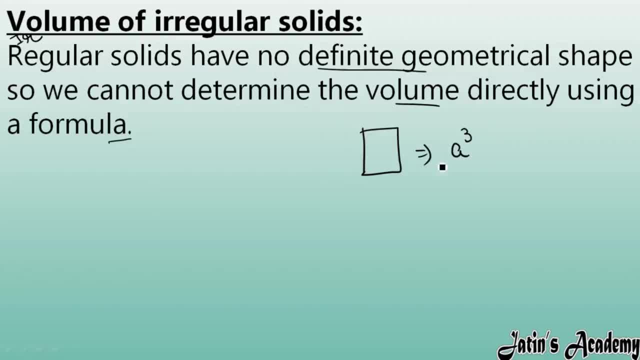 We are having one cube, that volume We are easily measuring side cube. If we are having cuboid, cuboid is a regular solid. We are using length into breadth, into height, these kind of thing. We can easily measure the volume. But if I am having this kind of volume, so how I will find? by using any formula, because I'm not having any kind of formula in order to measure this. 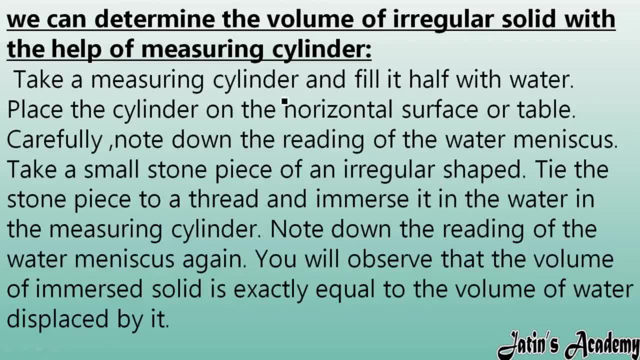 So how to measure this volume of irregular solids? here we are having so we can determine the volume of irregular solid with the help of measuring cylinder. Before only I have taught you about the measuring cylinder. So this is this: we are going to use measuring cylinder in order to measure the volume of irregular solid. 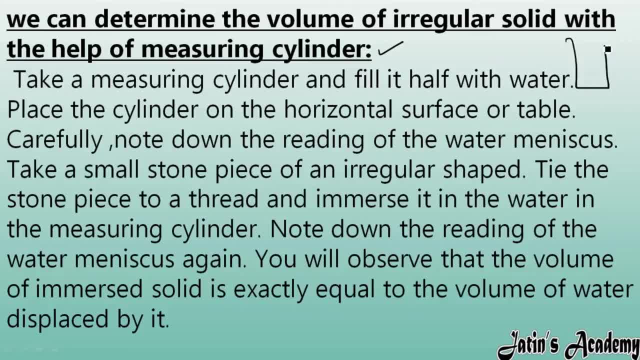 So what we have to do? we have to take a measuring cylinder here. We have to take a measuring cylinder and we have to fill half it with water, then fill half it with water. Now we have to place the cylinder on the horizontal place. horizontal place or horizontal surface table. 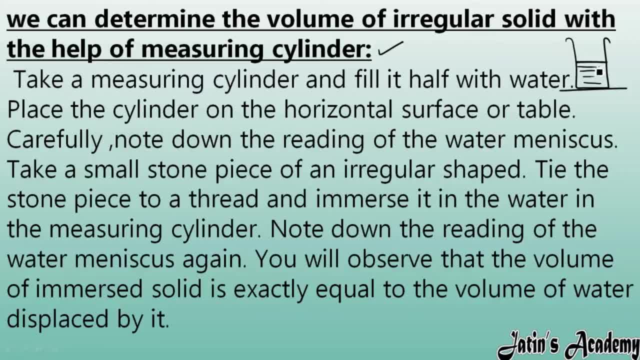 Now carefully note down the reading of meniscus, this reading carefully, We have to note. Okay, Then we have to take the small stone piece, For example, this stone piece, this volume of stone, I have to measure how much volume of stone is there. 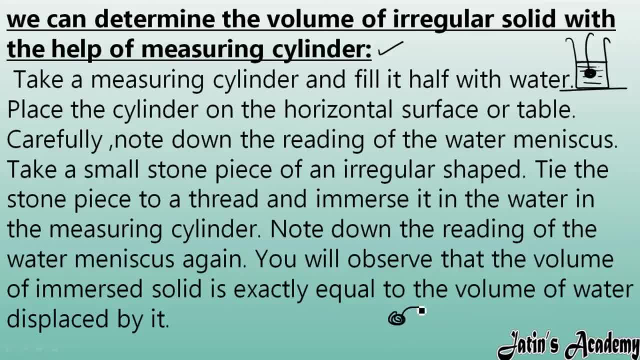 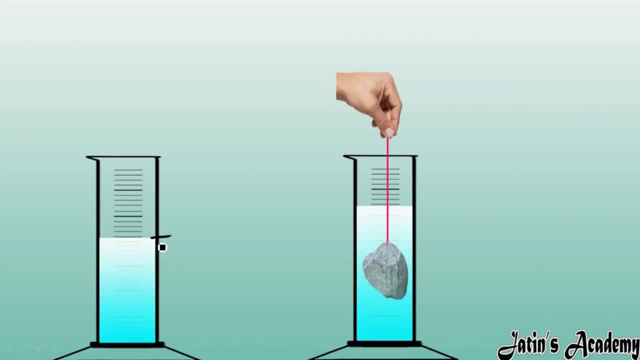 Okay, then we have to tie a thread. Firstly, take a stone and tie a thread on that stone and then gently immerse that stone that is tied with a string into a water- Okay, in a measuring cylinder. only then what we will see. we will see that, firstly, the volume of the liquid is still this: for example, this is 210 ml, but after: 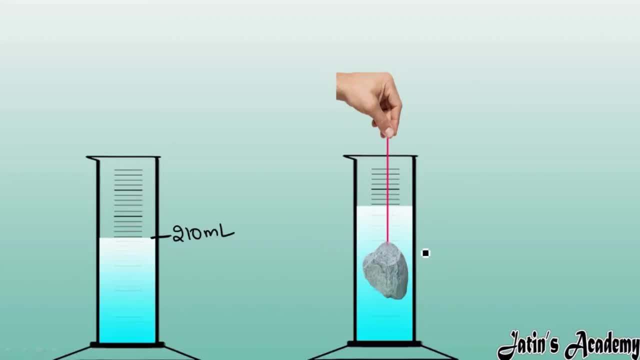 immerse the stone into it by using our thread, it will rise the level. the water level will rise and, for example, here it will 310 ml. Okay Now, in this case I want to measure the volume of this solid. So how will measure? I will just subtract the final and initial volume of liquid. 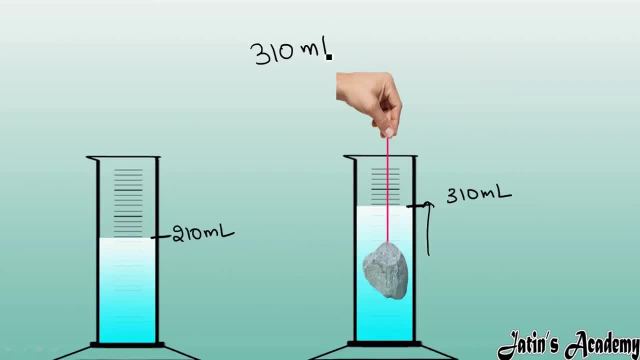 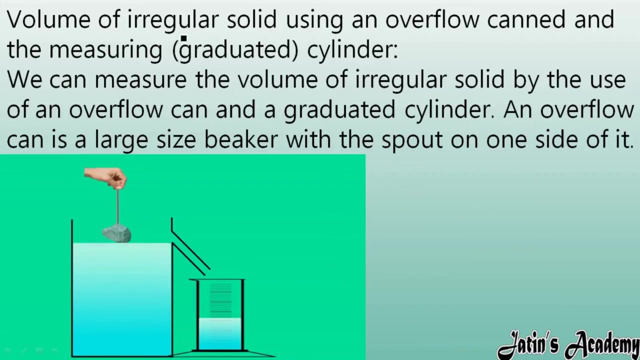 So final volume of liquid is 310 ml minus initial volume is 210 ml. So by subtracting what I will get hundred ml. fine, so means the volume of this irregular solid is what? 100 ml. this is the way how we can use graduated cylinder in order to know the volume of irregular solid. volume of irregular solid can. 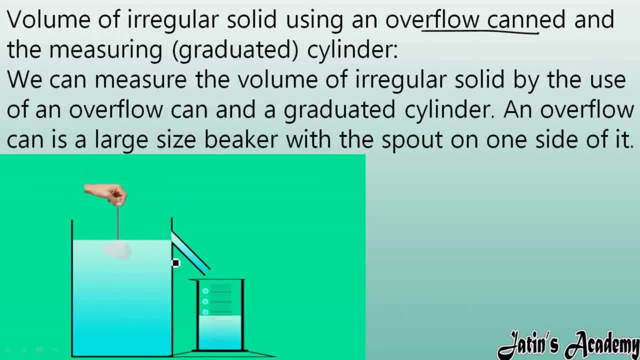 also be determined by using a overflow can. this is the overflow can, okay, or, and the measuring cylinder here. this: we are having overflow can, this is overflow can and this is measuring cylinder. so what we have to do, we can measure the volume of irregular solid. this volume of irregular solid. 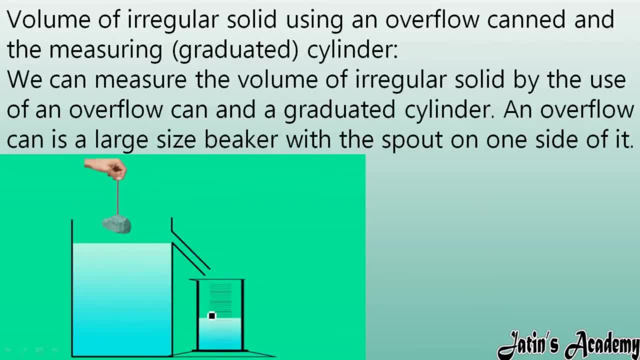 we can easily measure by using overflow can and measuring cylinder, how, for example, in this overflow can here till water is there, till here water is there and for example, 210 ml water is contained in this overflowing can. okay, then i will take one stone tied with a thread and i will gently 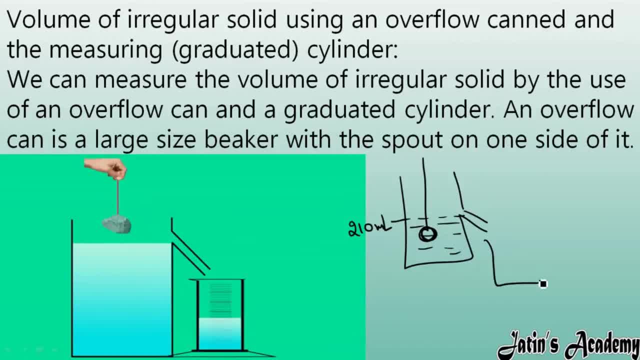 immerse into the overflow can then downside. i am having here measuring cylinder. so what we have to do, we can measure the volume of irregular solid, this volume measuring cylinder. so after immersed, after immersing the stone into this water, some kind of water level will come up and it will go down to the measuring cylinder. so while going down to the 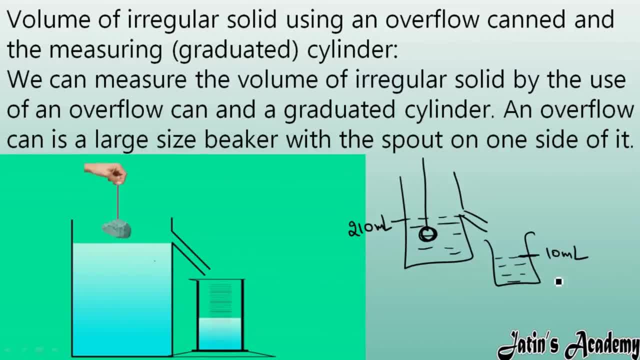 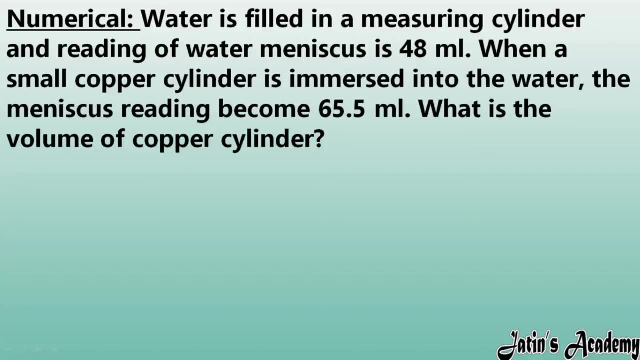 measuring cylinder, for example. here a 10 ml water came out. so this 10 ml of volume is nothing but the volume of this irregular solid. so how much amount of water came out, that much amount of volume is the volume of this irregular solid. next we are having numerical related to this. 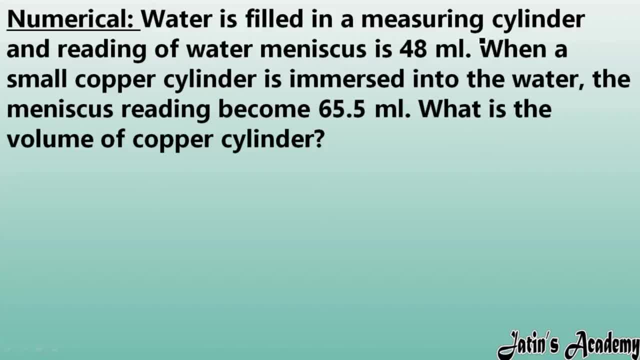 so numerical we are having. water is filled in a measuring cylinder and reading of water meniscus is 48 milliliter. so here, water is filled in a measuring cylinder and the when we are going to put the water in this measuring cylinder, water meniscus reading is till this water is filled. 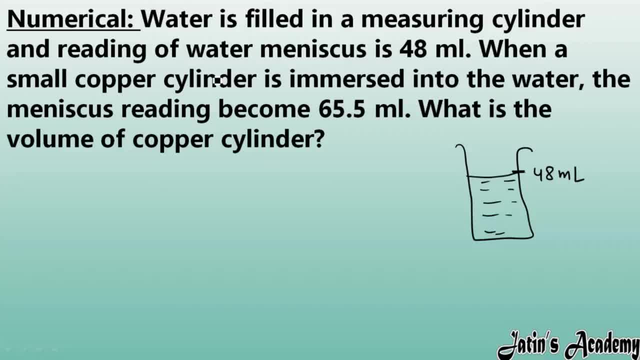 and this water meniscus reading is 48 ml. when a small copper cylinder is immersed into the water. when we are going to immerse small copper cylinder into the water, the meniscus reading becomes 65.5 ml. so this water level rises up and after rising this level reaches up to 65.5 ml. fine, so what is the? 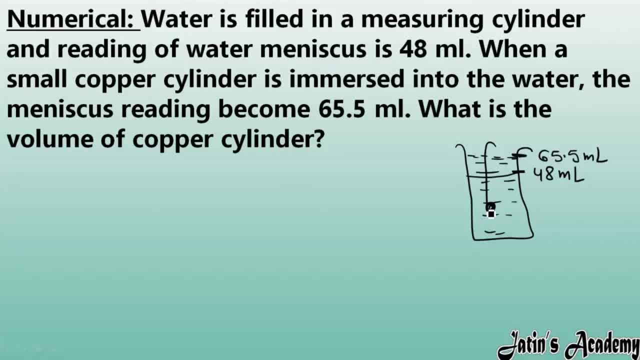 volume of copper cylinder. this volume of copper cylinder we have to find. so now only i have told: firstly we have to check the initial volume. initial volume: v1 is 48 ml. then we have to check the final volume. finally, we have to check the initial volume, we have to check the initial volume. 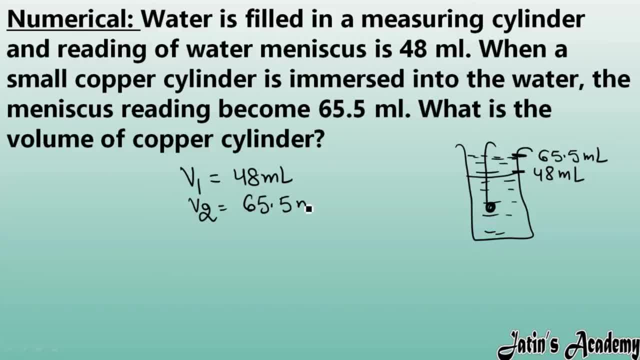 final volume, v2 is 65.5 ml. so for measuring the volume of this copper cylinder volume, volume of copper cylinder is equals to v2 minus v1. so what do you mean? what is the value of v2? 65.5 ml minus v1 is 48 ml. so after a subtraction, what you will get? you will get 17.5. 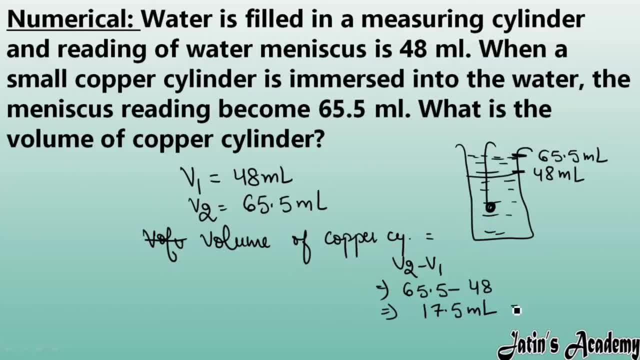 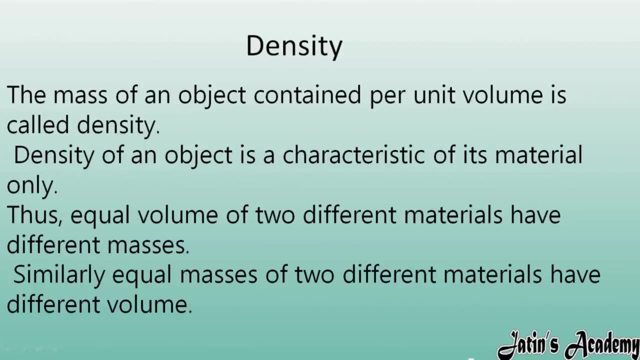 ml, if you want to write the answer in centimeter cube also, so instead of announcer the topic, density. so what do you mean by the density? the mass of an project contained per unit volume for educators, example, this much amount of volume I am having and in this volume how much mass is contained? 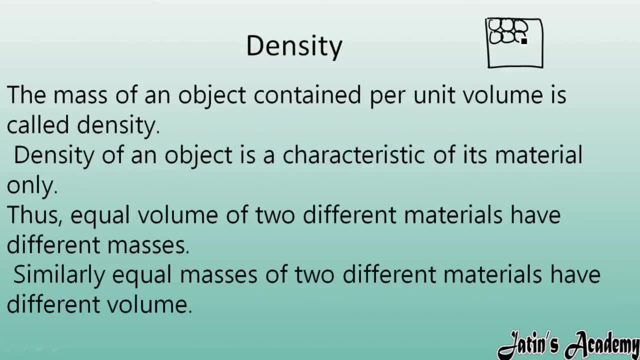 mass is nothing but matter how much mass is contained in this volume that is known as its density. okay, and density is a characteristic of material. only. density vary with material to material. it not going to depend upon shape and size, but it depends only upon the material. fine, 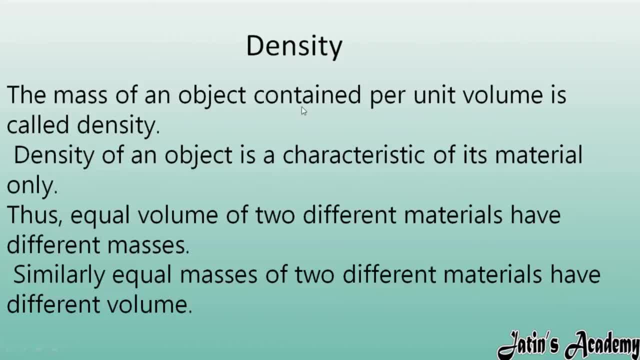 here it is written: does equal volume of two different materials have different masses? if, for example, here I am having cotton, this much cotton I am having, and this much gold I am having, for example, this is cotton and this is gold, this cotton and gold is having equal volume. okay, they. 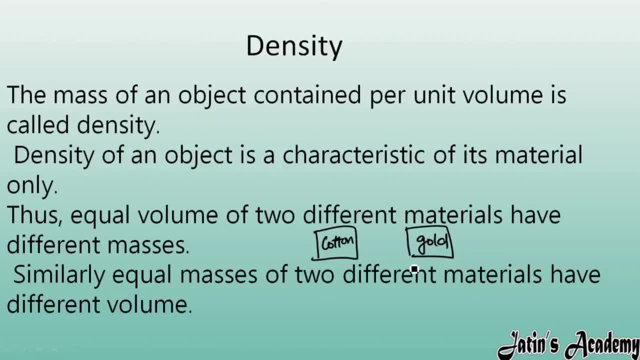 are having equal volume means space occupied by these. both materials are same, but mass of the subject is also same. one thing in one hand you can take cotton. in one hand you can take gold in the other hand. you just hold gold. so which among the following is heavier? obviously, mass of gold is. 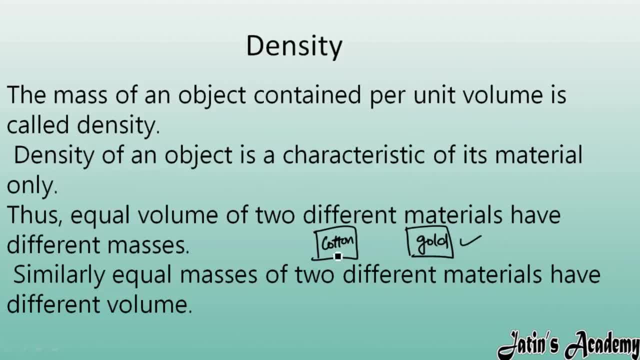 heavier as compared to cotton. so here if you are having to same volume also of different material but masses is going to different, fine, here. similarly, if I am having equal mass of two different materials, this much cotton I am having, for example, two kg cotton is there and this much. 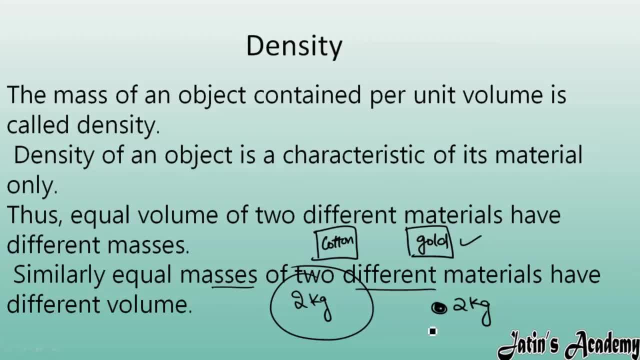 two kg gold is there, so they both are having same mass. but you can check the volume. volume is same. no, this much volume is same, so it is equal mass of two different materials and this much gold is same. so this volume is more because volume of the cotton is more as compared to volume of gold. so 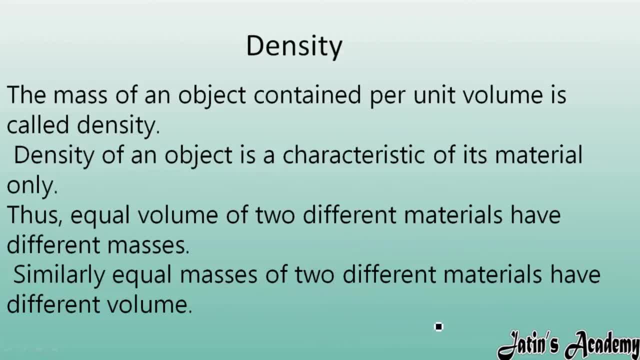 same mass is having different volume. so by this, what you will conclude? you will conclude that density is nothing but mass per unit volume. density. you can also write like this: rho, density is equals to mass per unit volume. and this relation, this formula, we are going to use. 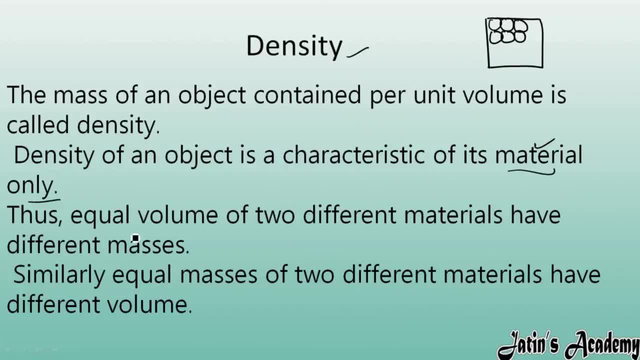 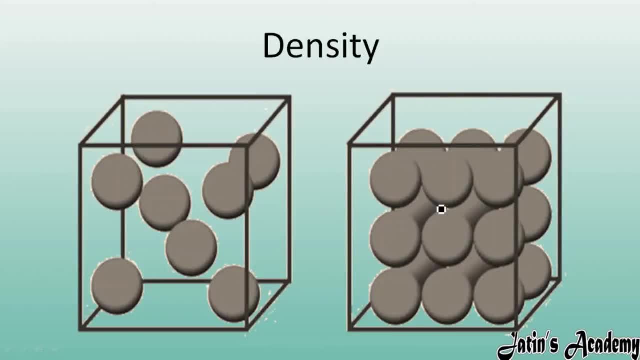 in order to solve the numericals. so here is a density. density is defined as mass contained per unit volume. so here is a density. density is defined as mass contained per unit volume. in this volume, how much matter is contained? that is defined as its density. Next, we are having units of density. 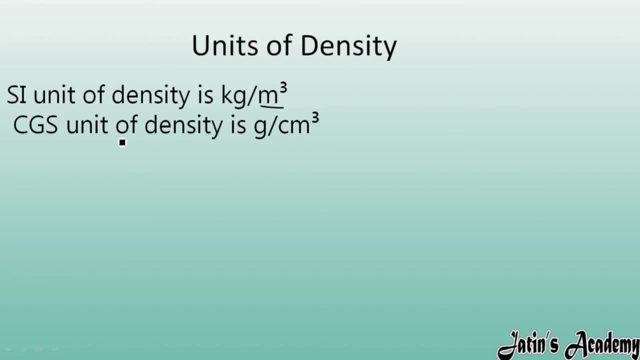 so SI unit of density is kilogram per meter cube and CGS unit of density is gram per centimeter cube. this you have to remember properly, fine. next we are having relation between SI and CGS unit of density. now we are going to do the relation between SI unit, that is, kilogram per meter cube. 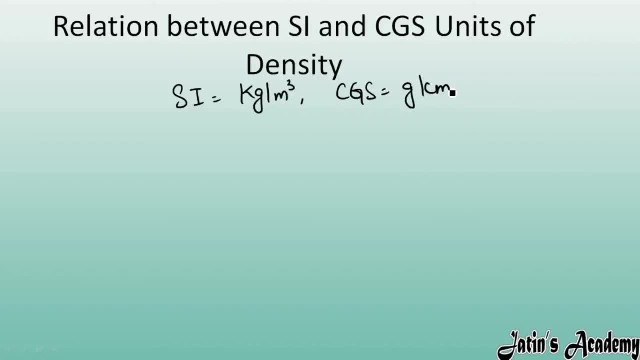 and CGS unit it. that is gram per centimeter cube, the relation between among them. we are going to do now. so can i write this one kilogram per meter cube as one kilogram over one meter cube, because here per means over divide. fine, and as you know, one kilogram is equals to how many gram, it is thousand gram. 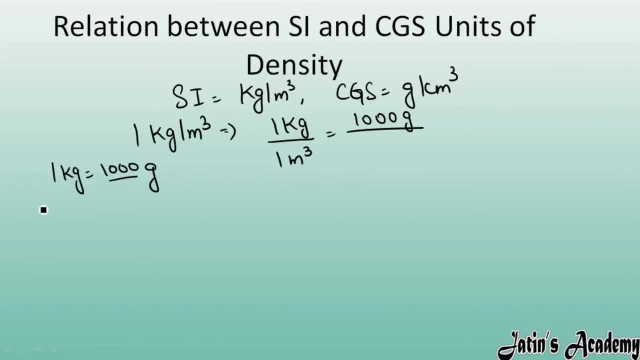 so one kg can i write thousand gram? and as we know, one meter is equals to hundred centimeter. fine, but here i am having one meter cube. one meter cube means one meter multiply one meter, multiply one meter. so instead of one meter i am going to put centimeter, so here it will be hundred. 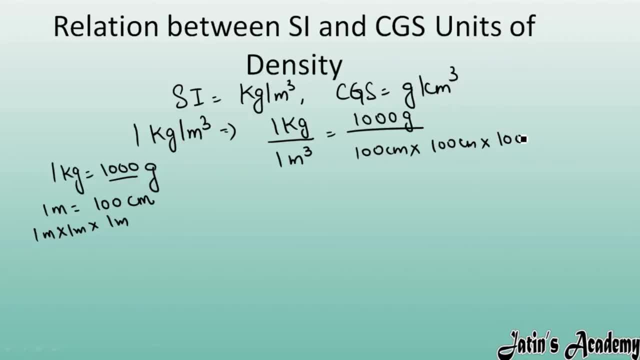 centimeter. hundred centimeter multiply hundred centimeter. why i am going to put by three? because here cube is there. that is why three values i have used. so here it will be. one kilogram over one meter cube is equals to one, two, three. one, two, three by simple calculation i. 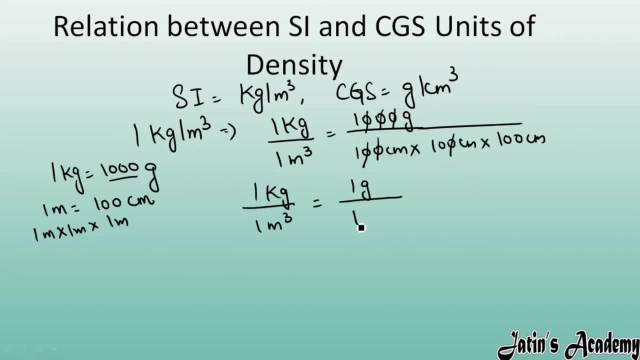 am going to cut the zeros, so here it will be: one gram over thousand centimeter cube. so can i write like this: one kilogram per meter cube is equals to one by thousand gram per centimeter cube. this is a relation between si and cgs, unit of density. and if this thousand 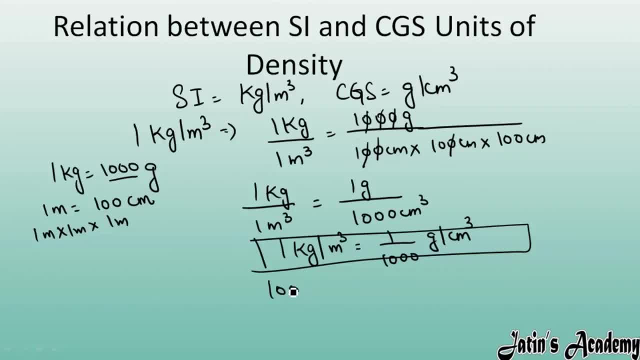 is equal to one by thousand gram per centimeter cube, then we are going to put one kilogram over is in divide. that side you can take in multiply also, so here it will be: 1000 kilogram per meter cube is equals to 1 gram per centimeter cube. like this or like this you can write the relation: 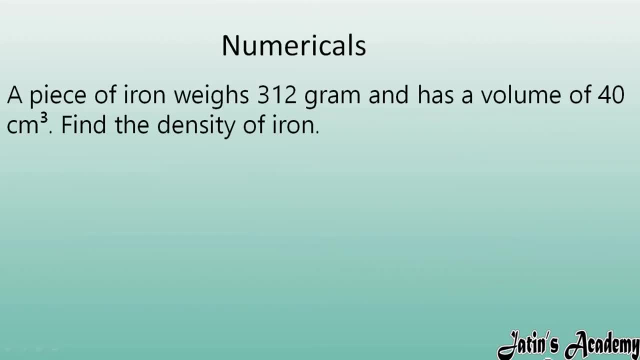 between SI and CGS unit of density. next we are having numericals. so first numerical we are having a piece of iron weighs 312 gram. so mass of iron is given to us. mass of iron is equals to 312 gram and has volume of 40 centimeter cube, and volume of iron is given to us that is 40 centimeter cube. 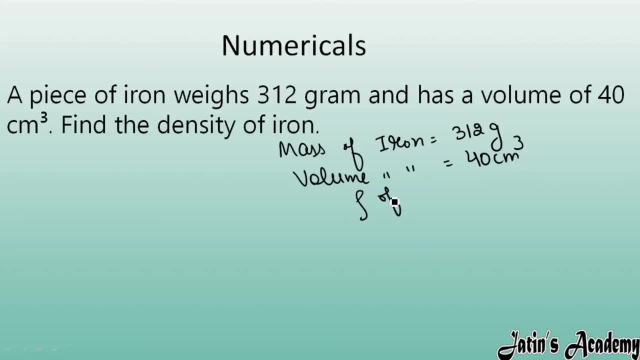 we have to check the density of iron. so density of iron we have to check. okay, so in order to check the density, first of all we are going to check the density of iron, we are going to check the formula: density is equals to mass over volume. but before using the terms into the numerical, into 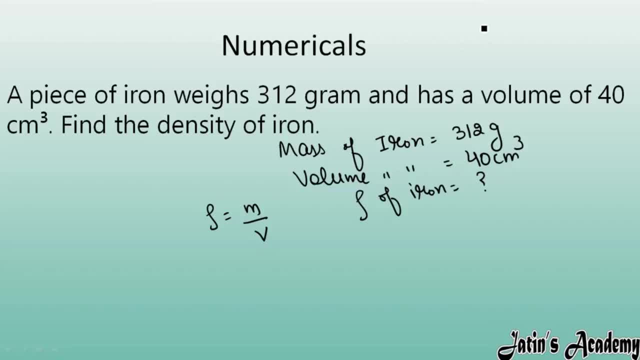 the formula. firstly check one thing: that, in order to check the density, firstly see that mass and volume is either given in centimeter cube or it should be in kilogram per meter cube. this units we have to check: either it is in CGS unit, either it is in SI unit. okay, now, here you can check mass. 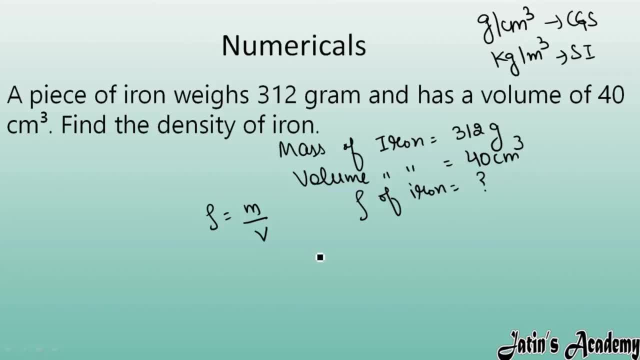 is in gram, volume is in centimeter cube and mass is in gram, volume is in centimeter cube. so now it's okay, just put the values. density is equals to mass, mass is what? 312 gram over volume is 40 centimeter cube. so your answer will be, after solving, 7.8 gram per centimeter cube. next, 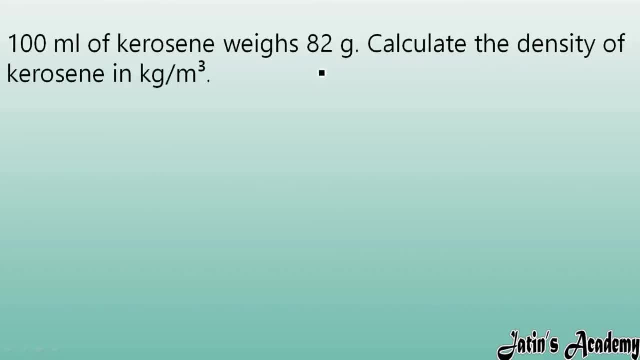 numerical we are having. 100 ml of kerosene weighs 82 gram. 100 ml means volume of kerosene is given to us. volume of kerosene is equals to 100 ml. so we are going to check the density of iron. we are. 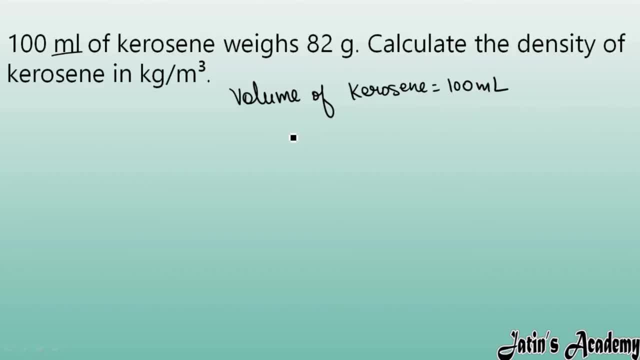 going to check the density of Centimeter iba. so, as we know, volume always we are using either in centimeter cube either in meter cube. just convert this milliliter into centimeter cube. as we know, one milliliter is equals to one centimeter cube. so volume of kerosene. you can also write it like: 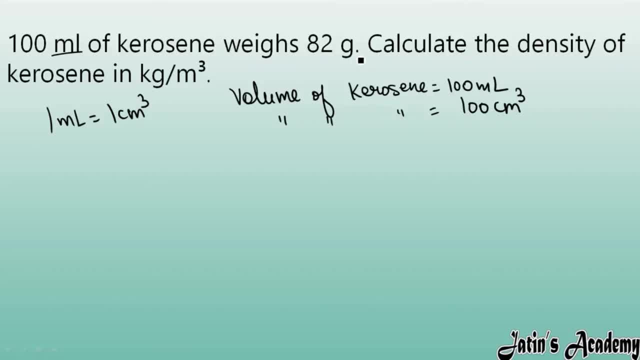 this and hundred centimeter cube weighs 82 gram. so here we are given with mass. so mass of kerosene is equals to 82 gram. find calculated density of kerosene in kilogram per meter square is also known to be a copおい. 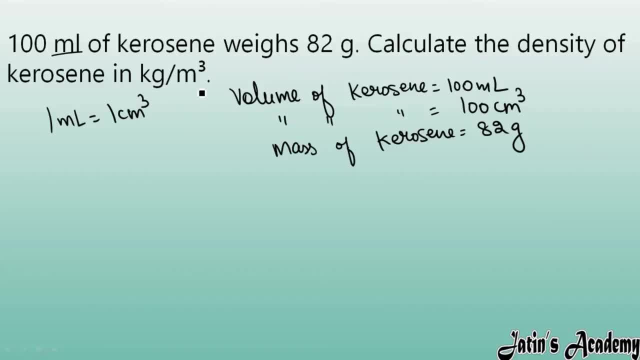 cube. so density of kerosene we have to check, but we have to check in kilogram per meter cube. so firstly calculate the density first of all. i am going to calculate the density in gram per centimeter cube only. after that i will multiply by thousand, okay. so density, we know density is. 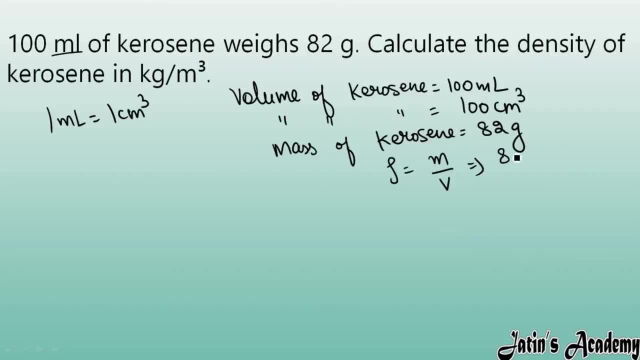 equals to mass over volume. so what is the mass of kerosene? mass of kerosene is 82 gram over volume is 100. okay, so after solving what you will get, you will get 0.82 gram per centimeter cube. here this answer is incomplete. why? because they ask the question in kilogram per meter cube. so just 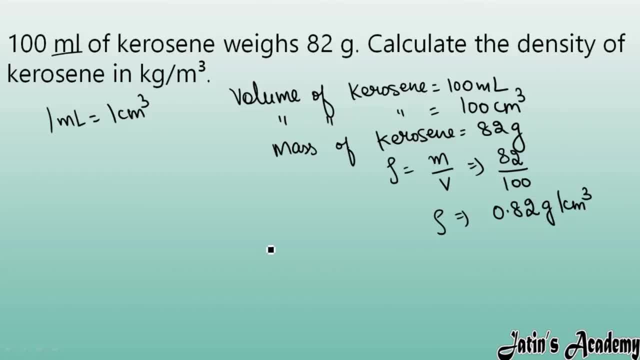 convert this gram per centimeter cube in kilogram per meter cube. so i am going to convert here 0.8. if question is like this: you have to convert gram per centimeter cube into kilogram per meter cube. just multiply the value you, this value with 1000. okay, and after that write kilogram per meter cube. so how you will write. 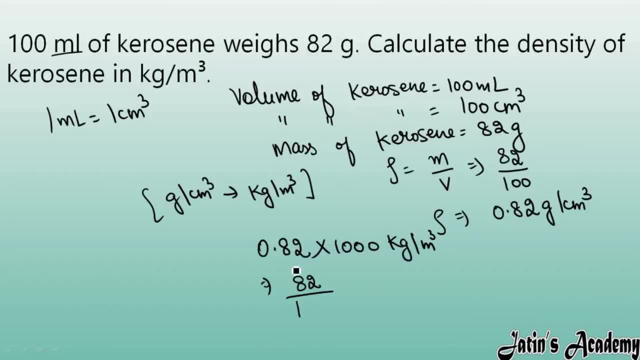 82 as such over. instead of point, i am going to write one after point. two digits are there, so two zeros will be there. multiply 1000, 0, 0, cut with 0, 0, so your answer will be 820 kilogram per meter. 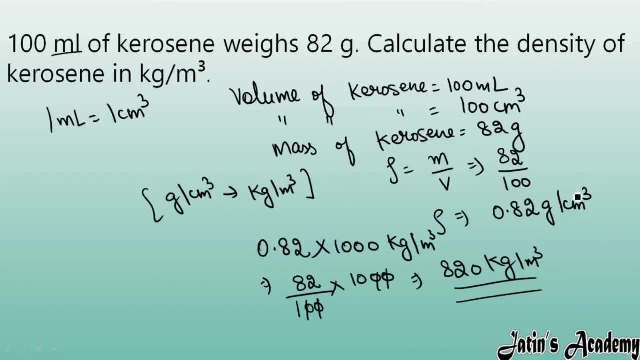 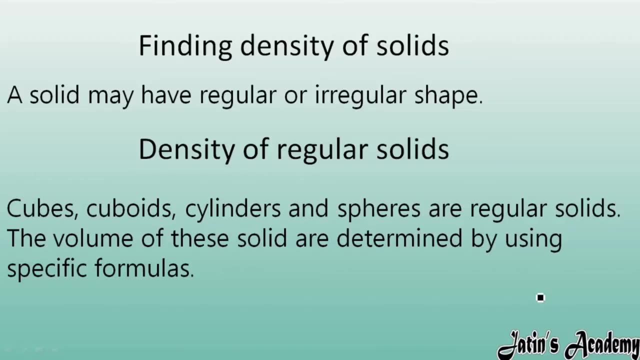 cube might be. you got the answer that when you have to convert gram per centimeter cube into kilogram per meter cube, just multiply this term by 1000. you will get answer in sa unit system. next we are having find density of solid. now how to find the density of solid? 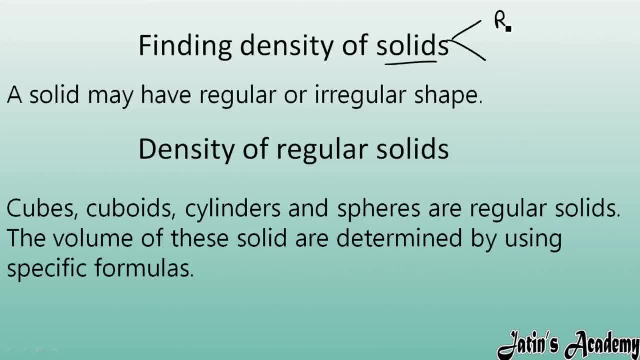 as we know, solid are of two types. solid out of two type, that is, regular solid and second we are having irregular shaped solids. so, one by one, we will study. firstly we will study about density of regular solids. so what are regular solids, like cube, cuboid solid, and then we will study about density of regular solids. so what are regular solids like? 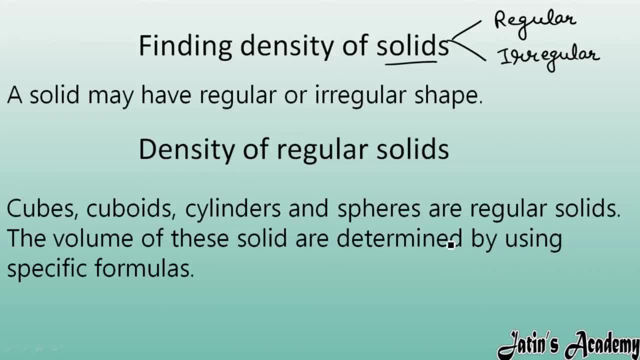 cylinder spheres. these all are regular solids and we know, as we know, density is equals to mass over volume. fine, so like, for example, here i am having cube, i want to measure the density of cube. so how to measure density of cube? by using formula: density is equal to mass over volume. 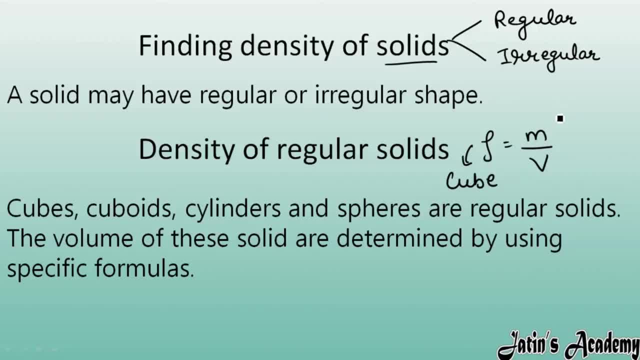 so mass of the volume, mass of the cube, i can simply measure by using beam balance. i will take the beam balance. okay, this kind of beam balance i will take and i will measure the mass of this cube. now the problem is about volume. volume is not that much problem because we know. 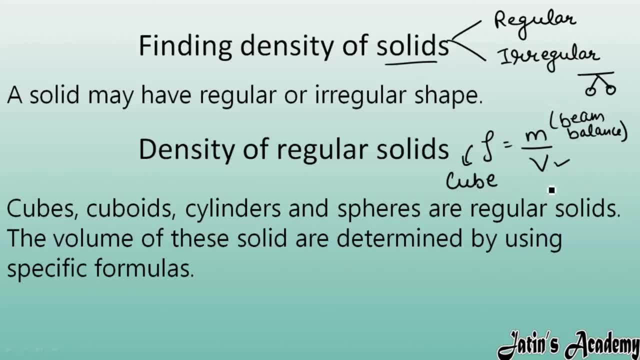 how to find the volume of cube. by using the formula, so simply we can find volume also. so by using the beam balance and by using the appropriate formula, we can simply calculate the density of regular solid. regular solid is not a matter, but matter is about the irregular solid. 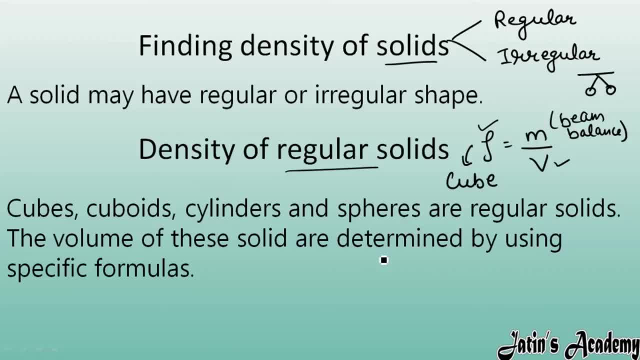 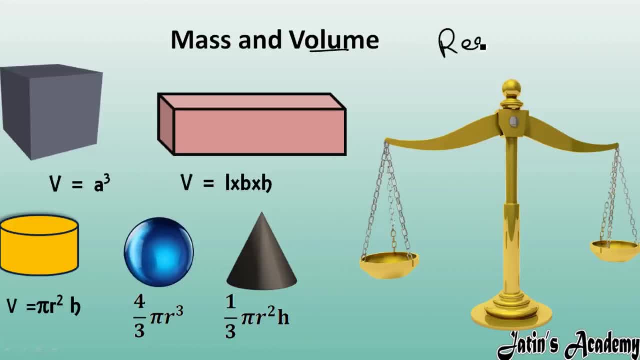 and the next slide we will study about the irregular solid also. firstly, we will see about the regular solids. so here we are having mass and volume. so mass of each and every regular solid, mass of each and every regular solid we are going to measure by using the beam balance. this is a beam. 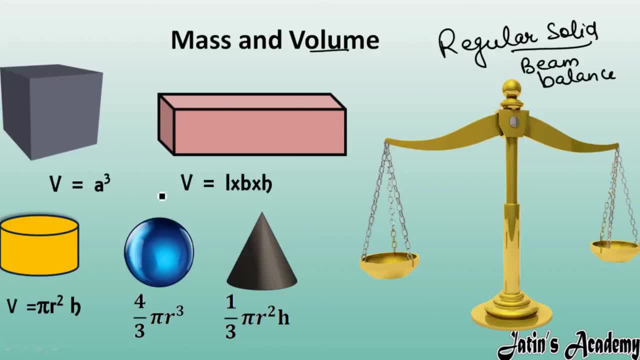 balance. so mass we can easily measure and volume we can easily measure by using appropriate formula. if i am having cube, i will use this formula. if i'm having cuboid cylinder sphere cone, i can easily measure any volume, any mass. fine. so by using the formula, density is equals to mass over volume. 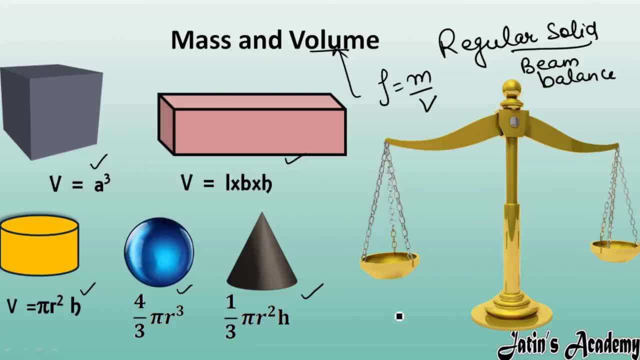 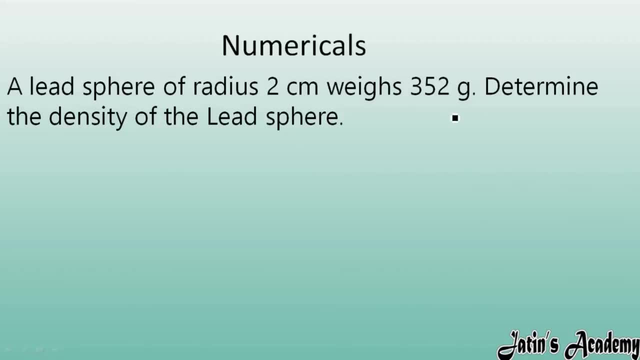 I can measure the density of any regular shaped object. Next, numerical, we are having a lead sphere of radius 2 centimeter weighs 352 gram. So here we are given with a lead sphere. So this is a, for example, lead sphere which is having radius 2 centimeter and mass of 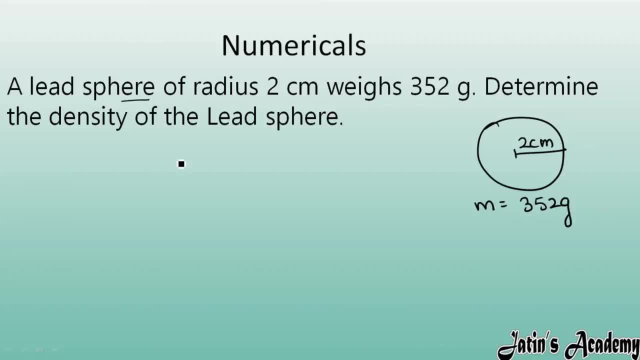 lead sphere is given 352 gram Determine the density of lead sphere. So density of lead sphere we have to calculate. So how to calculate density? So we know density is equals to mass over volume. So density of lead sphere we have to calculate. 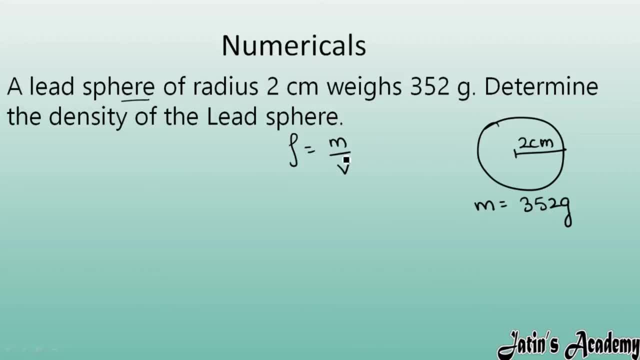 Mass of lead sphere is given. fine, but problem is of volume. So how to calculate the volume of sphere? So, as we know, the formula volume of sphere is nothing but 4 by 3 pi r cube. Okay, so 4 by 3 pi means 22 by 7 over r cube. 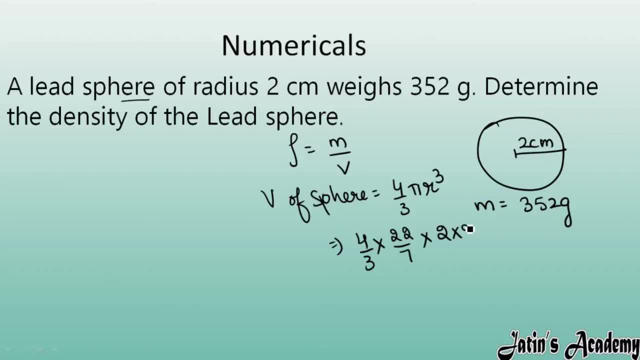 R means radius cube. Radius cube means 2 multiply 2.. After solving what you will get here, you will get the answer 704 by 21 centimeter cube. So volume we have found. now I am going to put the values in this formula. 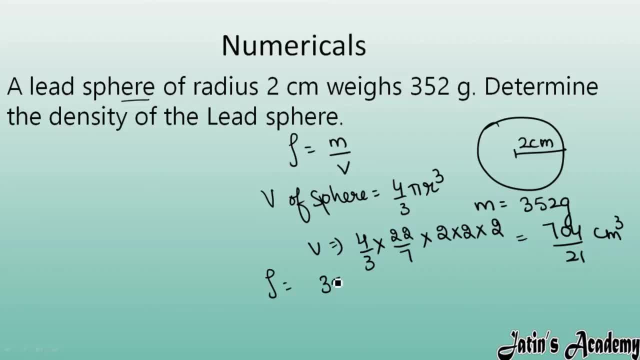 So density is equals to mass. Mass is what 352 divide. we have to do volume. So volume is 704 by 21.. So here I am going to write upward: density is equals to 352.. Instead of divide can I write multiply and after that I will reciprocal the next term. 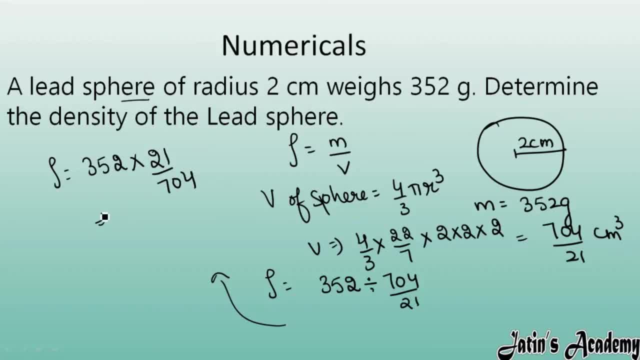 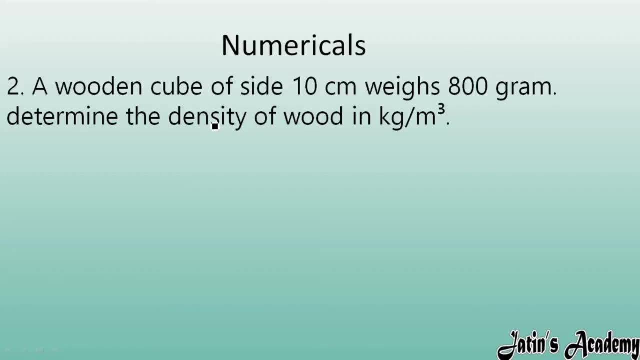 So just reciprocal, the next term. So what you will get after solving each and every calculation? you will get the answer: 10.5 gram per centimeter cube as the density of lead sphere. Next numerical: we are having a wooden cube of side, 10 centimeter weighs 800 gram. 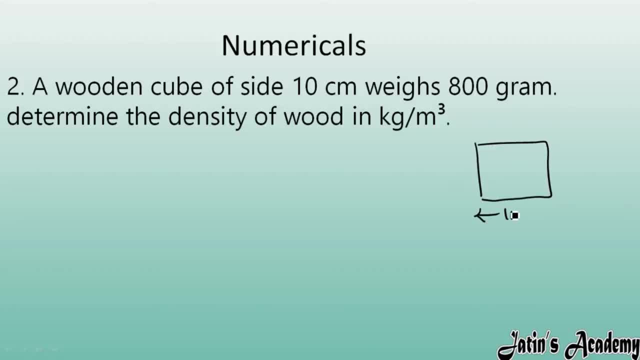 So here wooden cube is there which is having side 10 centimeter, weighs 800 gram. Weighs 800 gram means mass is given 800 gram Determine the density of wood in kilogram per meter cube. They have asked the density in SI unit system. 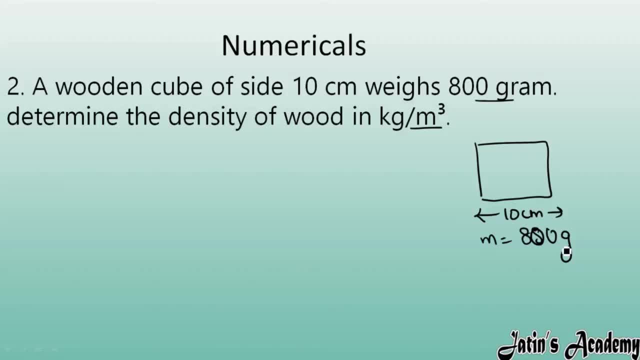 But quotient is given in gram, and centimeter means in CGS system. So firstly I will calculate the density in gram per centimeter cube. After that I will multiply with the thousand, So density. we know density is equals to mass over volume. So mass is what? 800.. 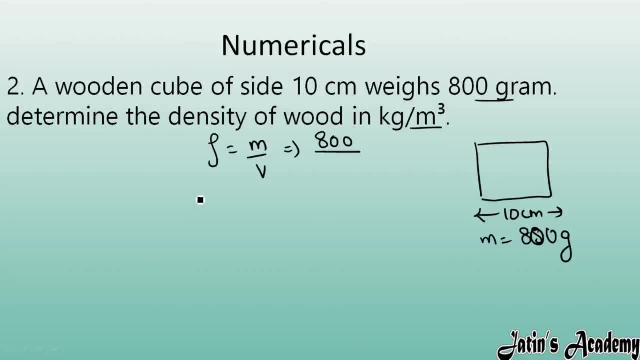 Over volume. volume volume we have not given of cube, just we have to find the volume. So volume of cube. volume of cube is equals to side cube. side cube means 10 cube, because side we have given 10.. So it will be 10 multiply 10. multiply 10, that is thousand centimeter cube. 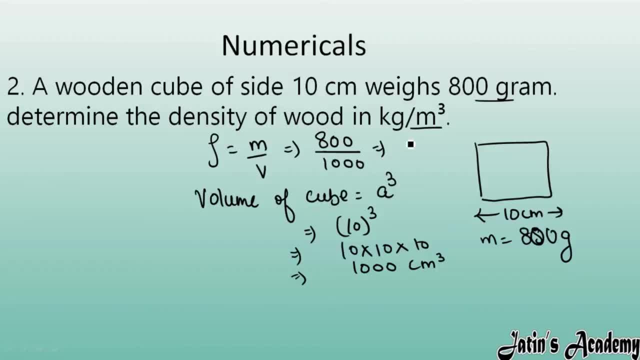 So volume is thousand centimeter cube. after solving what you will get 0.8 gram per centimeter cube. But they were. they have asked the question in kilogram per meter cube. So I have already told you. just take the value and multiply it by thousand kilogram per meter cube. 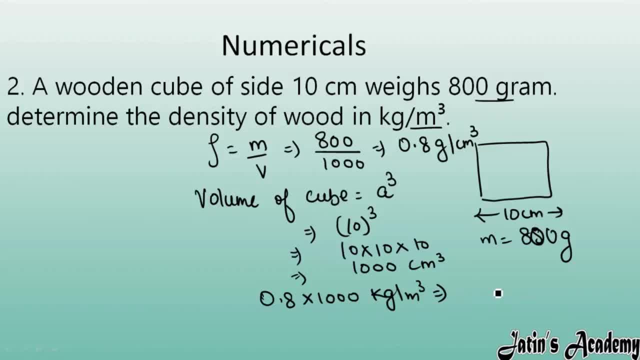 You will get the answer in kilogram per meter cube: 0.8.. Can I write it like this: 8 by 10 multiply thousand, as such kilogram per meter cube as such, 0, cut with 0.. So you will get the answer: 800 kilogram per meter cube as the density of wood. 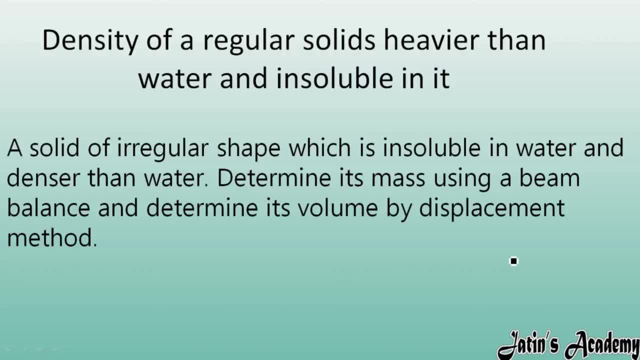 Next, we are having density of regular solid, heavier than water and insoluble in it. Actually, here we are having density of irregular solid. Here it is Irregular solid because regular solid vehicle we are going to find by the volume and mass. that is easy. 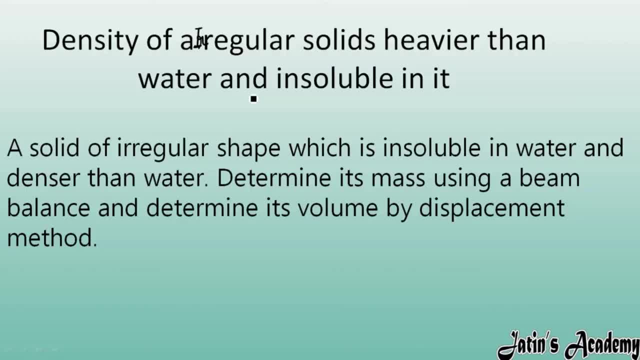 But problem is about irregular solids, So density of how to find the density of irregular solid which is heavier than water and insoluble in it, So mass. as we know, density is equals to equals to mass over volume. so mass, so we can easily find by using the beam balance, okay, mass. 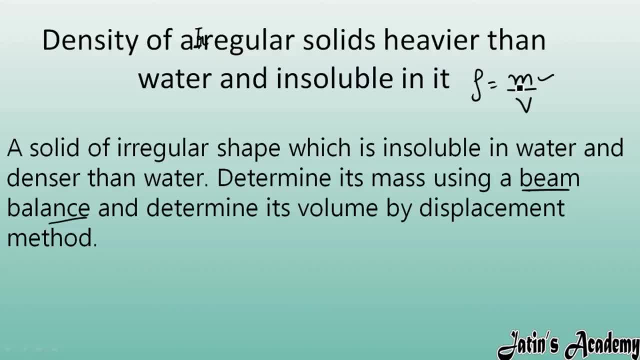 of any regular or irregular solid we are easily going to find by the beam balance. but problem is about the volume, because irregular solid we are not going to use any formula for irregular solid. so how to find the irregular solid volume? by using water displacement method. what is that? 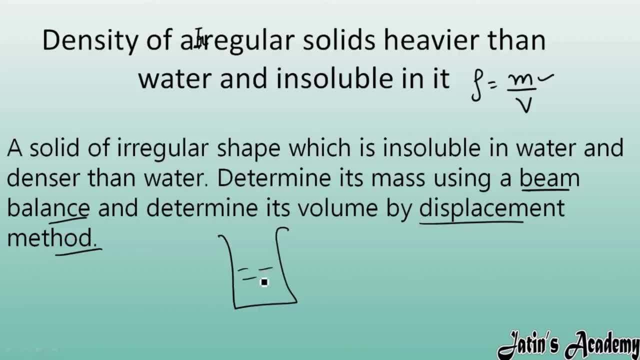 water displacement method. here we have to take measuring cylinder, put any kind of stone or any kind of irregular solid. then water level is going to rise, might be. now you got the answer. so here, whatever answer will come, and whatever, here initial reading will come by subtracting. 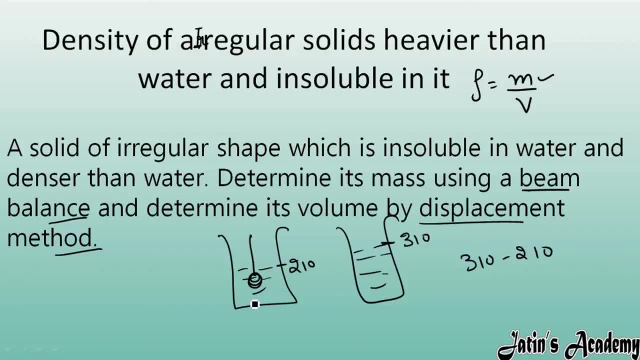 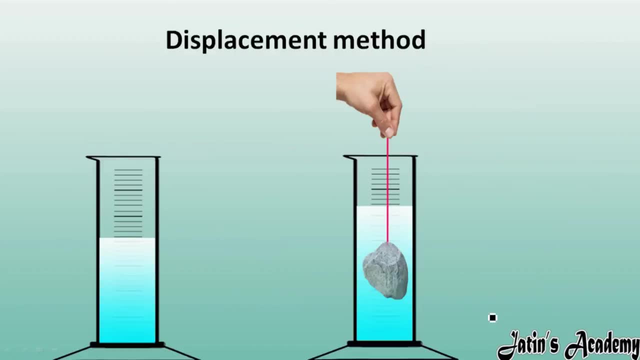 you will get the volume of this stone or irregular solid. so by this way, by this is known as liquid displacement method. so by this liquid displacement method, you can find the volume, fine and mass. you can find by using the beam balance. this is liquid displacement method. you can find the volume, fine and mass you can find by using the beam balance. this is liquid displacement method. you can find the volume, fine and mass you can find by using the beam balance. 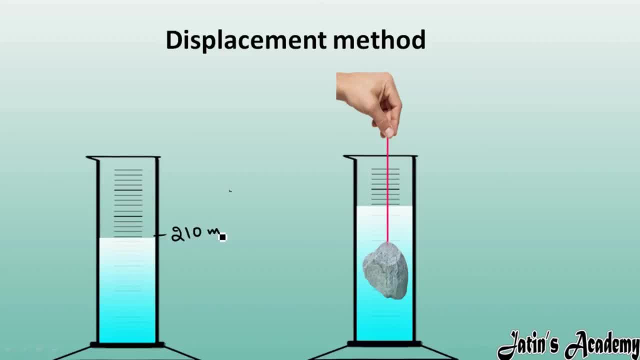 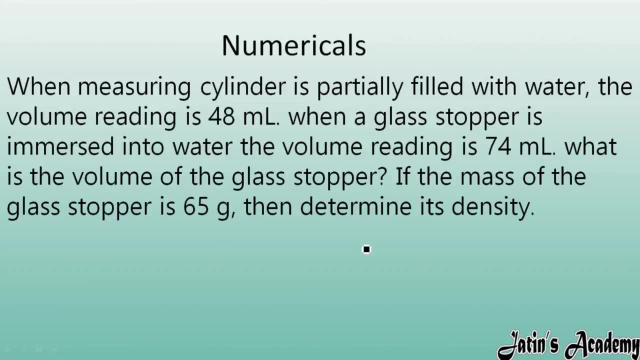 you can also remind: now, this is 200, for example, this is 210 ml, this is 310 ml. so by simply subtracting it we can calculate the volume of this irregular solid. next, we are having numericals related to this. so first, numerical we are having when a measuring cylinder is partially. 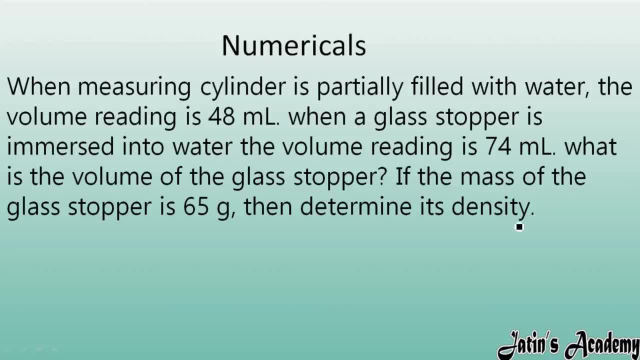 filled with water, the volume of reading is 48 ml. when we are having measuring cylinder and this measuring cylinder is partially filled with water, then its volume is 48 ml. when a glass stopper is immersed into it, when i am going to immerse the glass stopper into it, 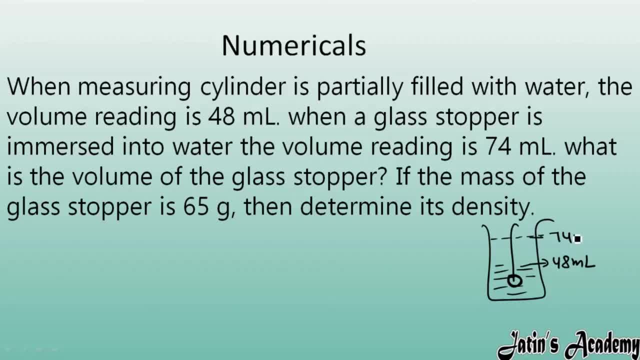 the volume of reading is going to rise and now it will be 74 ml. what is the volume of glass stopper? what is the volume? firstly, initial volume of water: we are having 48 ml. final volume of water: we are having 74 ml. so, in order to check the like volume of this glass stopper, we are just going to 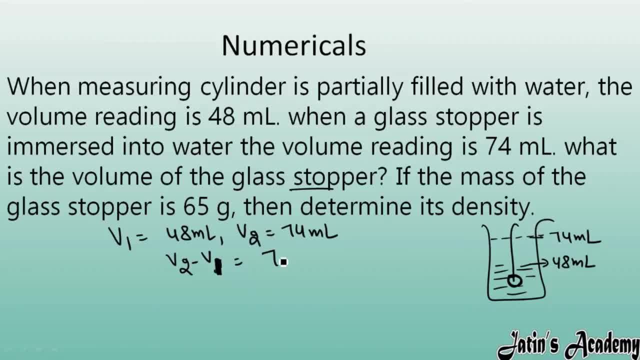 simply mine. we are going to subtract this volume, so 74 minus 48 it will give you 26 ml, and 26 ml is a volume of this glass stopper. or you can write 26 centimeter cube also, if the mass of the glass stopper is 65 kg. now we are given with 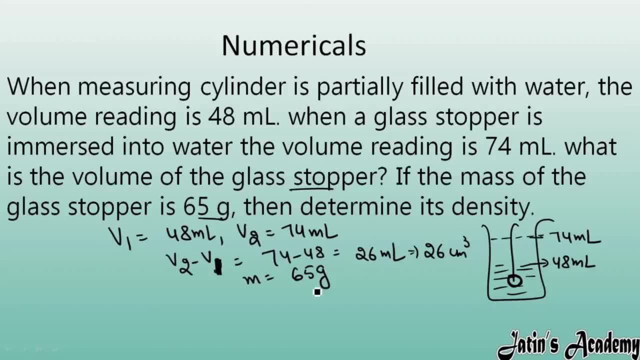 mass. also 65 gram determine its density. density we have to calculate. we know density is equals to mass over volume. mass we have given volume, we have calculated by using the formula here you will get 2.5 gram per centimeter cube. you can simply measure the density of any irregular solid. 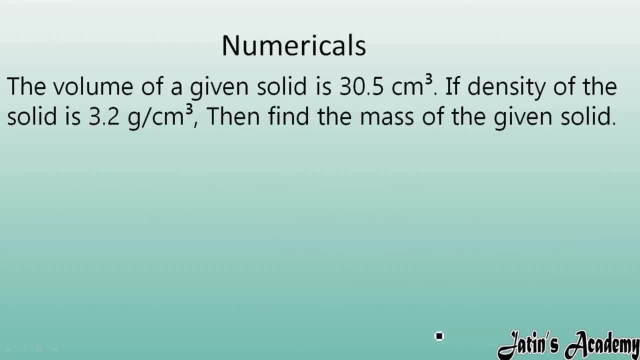 next numerical we are having: the volume of the given solid is 30.4 centimeter cube. here we are given with volume of solid, 30.5 centimeter cube. if the density of solid is this, now here we are given with density also 3.2 gram per centimeter cube- find the mass, mass we have to calculate. 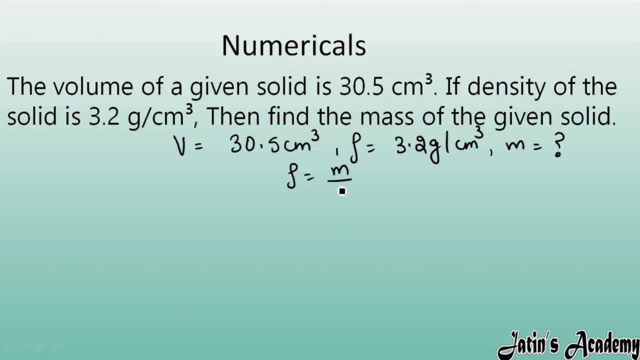 now you have to use the formula: density is equals to mass over volume. mass is nothing. so here just put the values. density is what 3.2 masses we have to find. volume is 30.5, so 30.5 is in divide. take that side in multiply, so 3.2 multiply 30.5 is equals to mass. so after multiplication what you 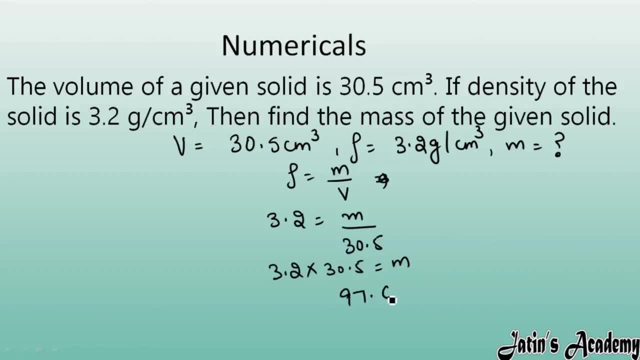 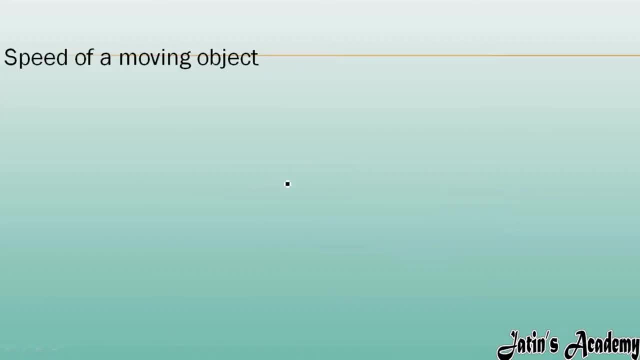 will get. you will get 97.6 gram as the mass of the glass stopper. so this is the mass of the glass stopper, the mass of this given solid fine. so next we are having speed of a moving object. so what do you mean by speed of a moving object? distance covered by a moving object in unit time. how much distance? 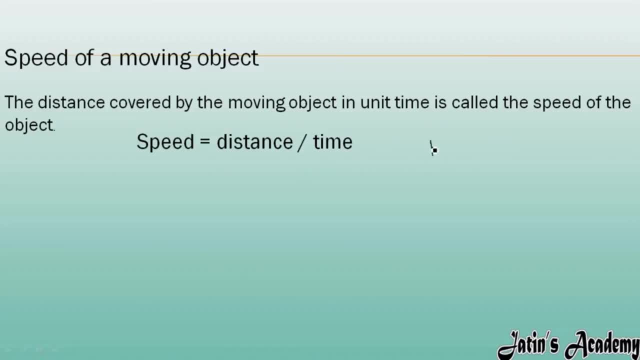 object has covered in how much time, for example, this is the object, so this much distance that object has to cover in a time in particular, time, so that distance over time will give you speed. so distance covered by a moving object per unit time is known as its speed spade. 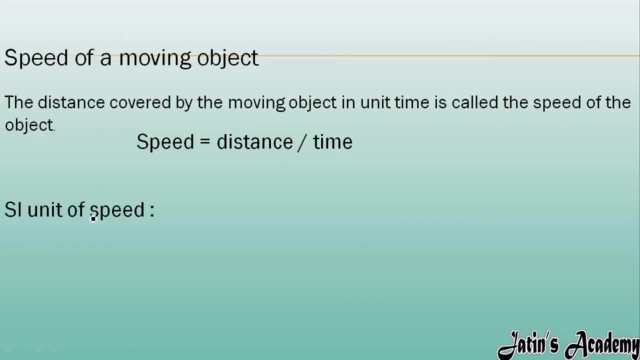 is equals to distance over time. now we are having a further unit of speed. we are going to calculate the SI unit of speed. so we know hear: SI unit of distance. firstly we will see the SI unit of distance. so SI unit, distance is what meter? and SI unit of time is second. ok, so we will see firstly, SI, unit of distance, right here. so here we have티s included in the time group dimension table, so there will be a distance added. next, I have to do something above the end, me and I profit, as you can see that now we have to add some. 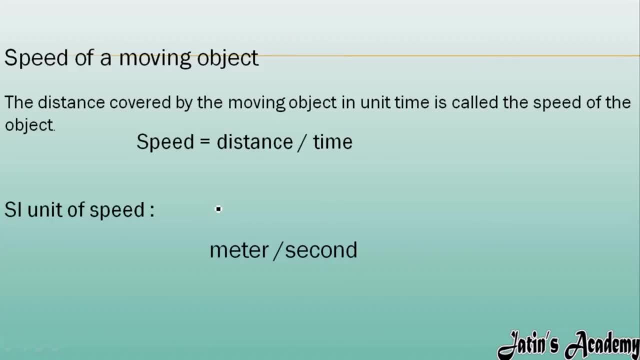 or less than what we have added. so we have to add other abilities. two: you can see that of distance, then we will see SI unit of time. so now the SI unit of speed is meter per second. you can write like this also. you can write like this also: SI unit of speed is SI unit of speed is meter. 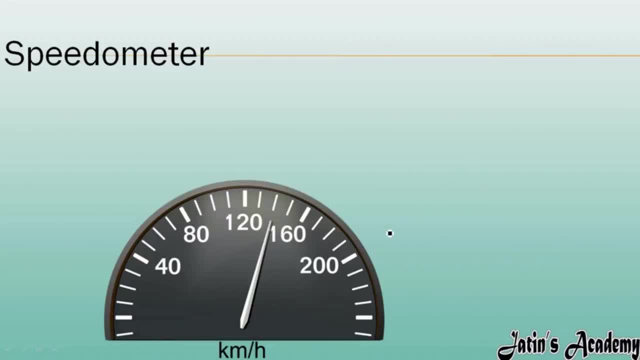 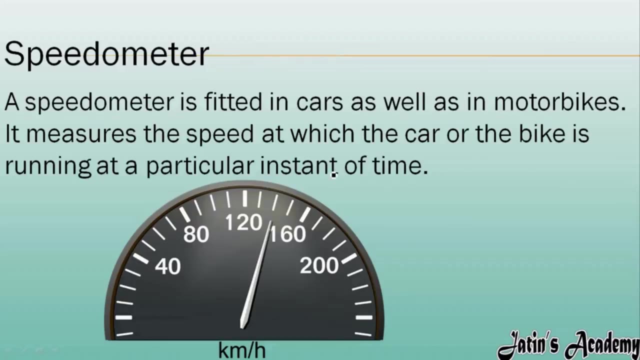 per second. fine. next we are having speedometer. might be you have seen this kind of instrument installed in our like activas or installed in our car. so what do the? what do you mean by the speedometer? speedometer is a fitted in car as well as in motorbikes. actually, speedometer is: 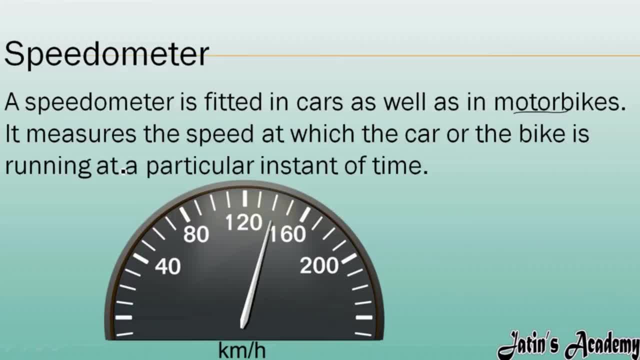 a device that is used in a car or bike to check the speed of a car, speed of the running car at a particular instant of time. so speedometer is fit in the car as well as motorbike and it measures the speed of car or bike at particular instant of time, like, for example, i am riding my 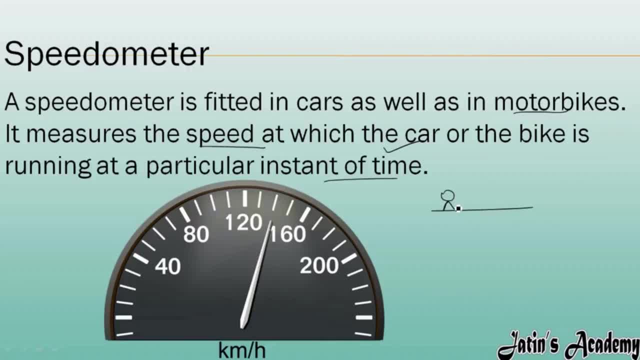 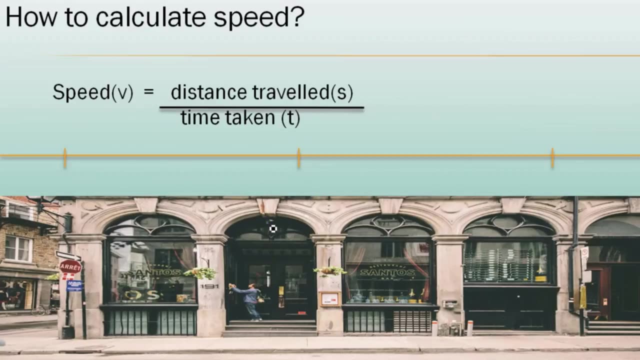 activa and i want to see what, at what speed, i am going. so to check, in order to check at what speed i am going, i will see the speedometer. so speedometer will give me the reading that at what speed my activa is going. fine, how to calculate speed. so we have already discussed the formula of 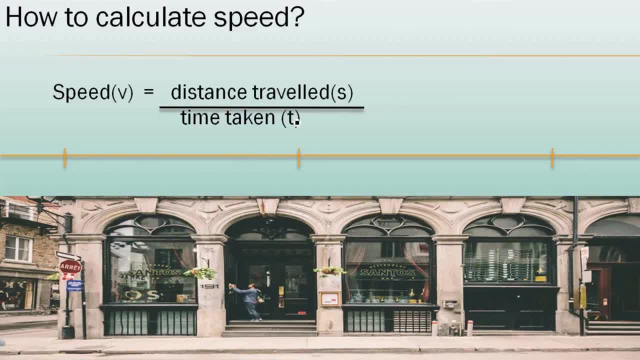 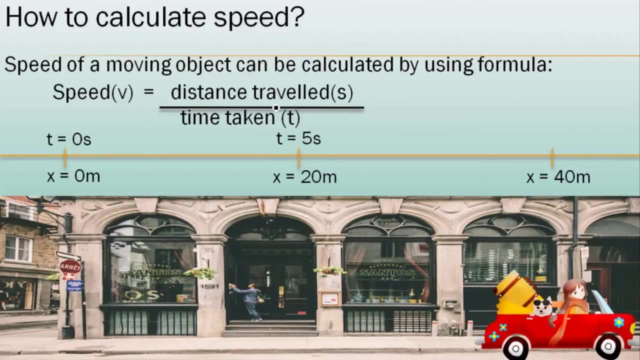 speed. that is, speed is equals to distance upon time. so by this formula we can easily calculate the speed of the car. and then this car is moving Hosted at the point c. that is the speed of the vehicle. and this car is moving on point a. afterwards it moves toward point b, then again it moves toward. 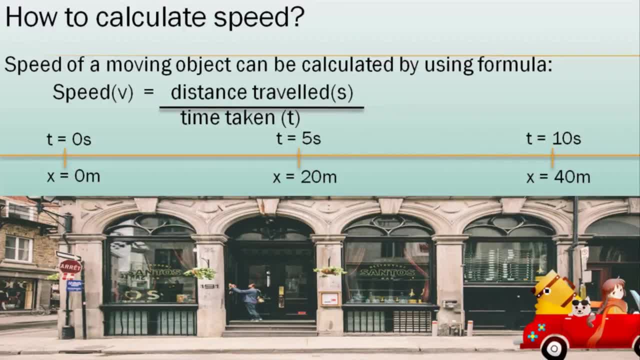 point c. so at this point c i want to check that. what is the speed of this car? fine, so what is the speed? actually, speed is distance over time, how much distance this car has covered. so this car has covered by speed. Speed equals to distance. Distance, that is, 40 upon time, Time is 10.. So speed, 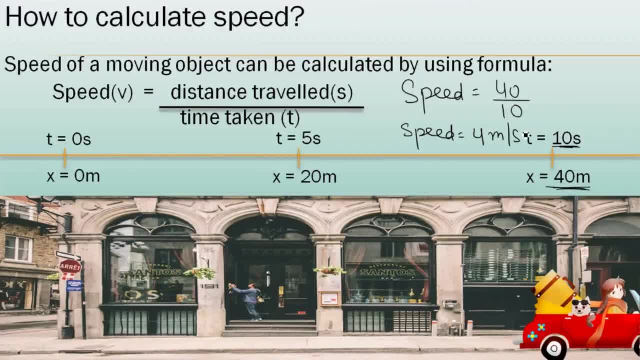 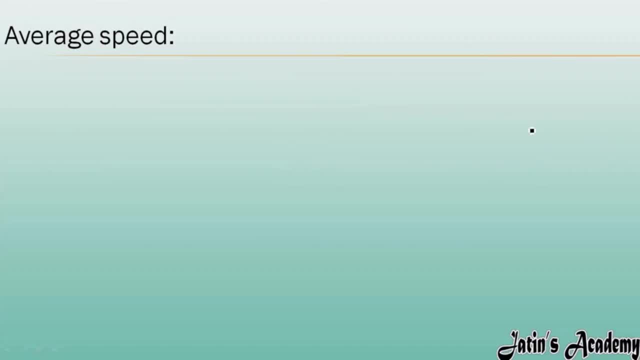 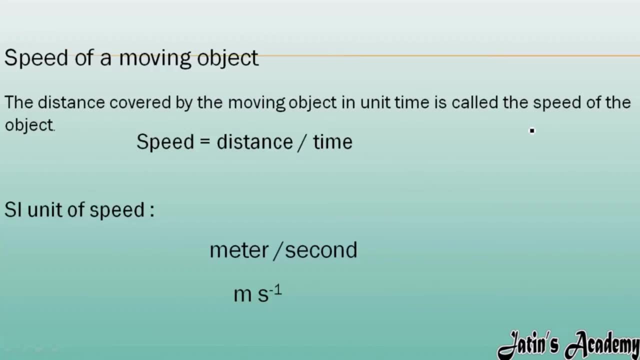 of this car is 4 meter per second. Clear Speed of this car is 4 meter per second. One thing more in this speed topic: Here we have discussed about the SI unit of speed. Here I want to tell you about the CGS unit of speed, also CGS unit of speed, So see how to calculate. 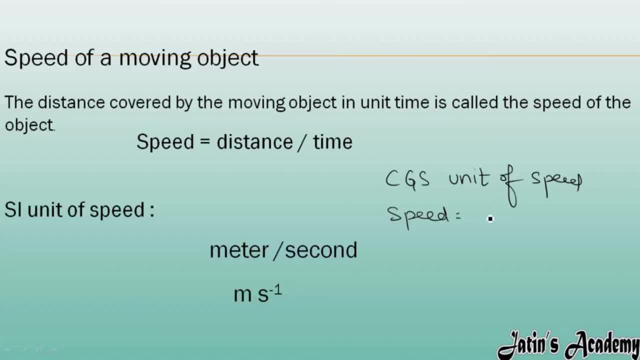 CGS unit of speed. We know speed equals to distance upon time. Fine, So here distance is what In CGS actually we are having. C means centimeter, G means gram and S means second, S means second. Okay, So here we want to. 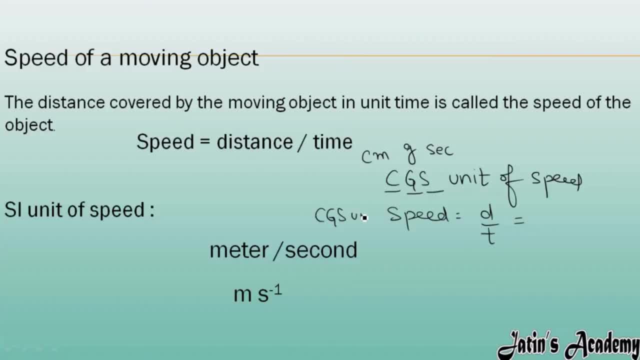 check the CGS unit of speed, CGS unit of speed. So tell me what is the CGS unit of distance? CGS unit of distance is centimeter And CGS unit of time is second. So CGS unit of speed is centimeter per second. What is the SI unit Meter per second? What is the? 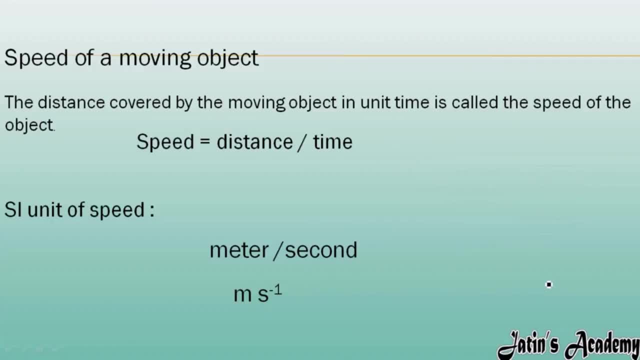 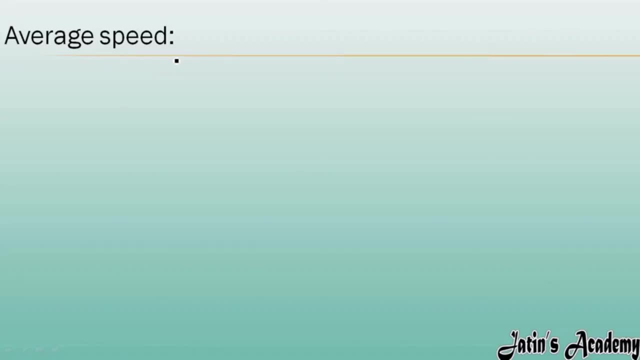 CGS unit Centimeter per second. Fine, So this we have already done. Next, we are going to start with the next topic, that is average speed. So what do you mean by average speed? Actually, whenever we are riding our Activa, we are on our car, the 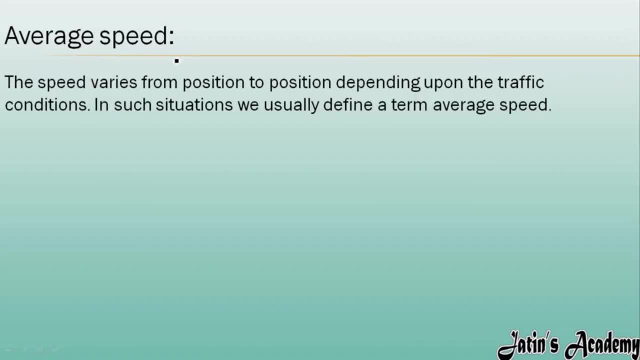 speed is not same or we are not covering same distance in same time. Why? Due to, might be some traffic conditions, we are not able to cover same distance. So sometimes speed is going to vary. Varies means changing from. Speed is going to change from position to. 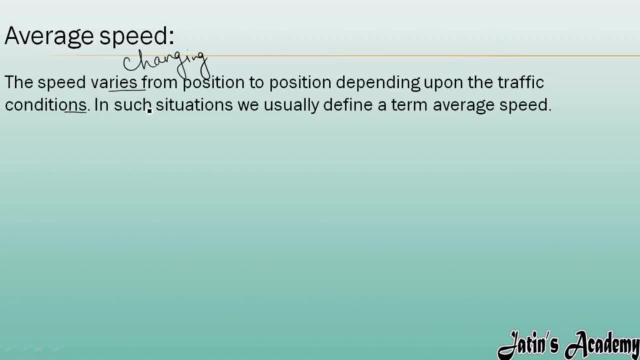 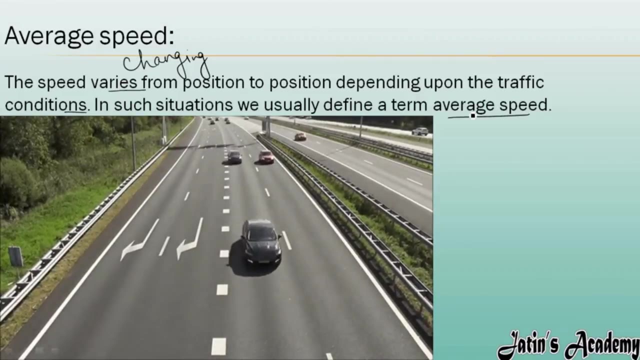 position. So in this situation, we are not going to see the speed. In this situation we are going to see the average speed. Fine, So here for example, see, due to this traffic and all this, these all cars are not having their same speed, So their speed is varying from position to. 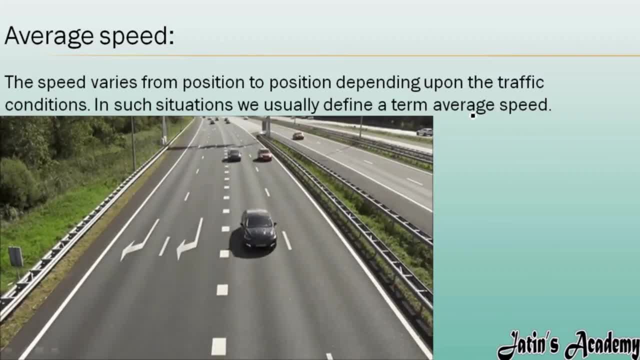 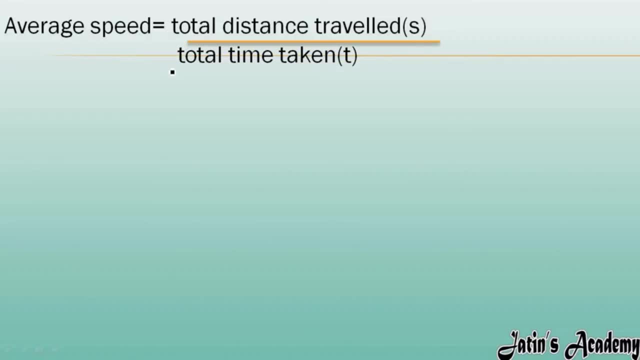 position that is known as its average speed. Now see the formula for average speed. As we have learned for the speed, speed is equals to distance upon time. Now we will see the formula for average speed. Average speed is equals to total distance. 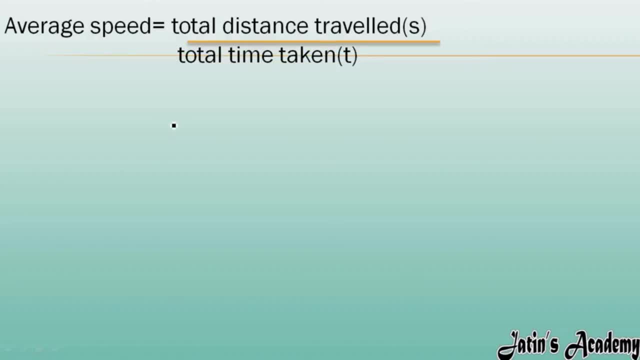 travelled over total time taken. For example, firstly this car is here, It took, for example, 5 seconds for 10 meter. Then it took again 5 second, for example, 25 meter, due to no traffic condition it going to cover more distance. So accordingly, we are to see the different. 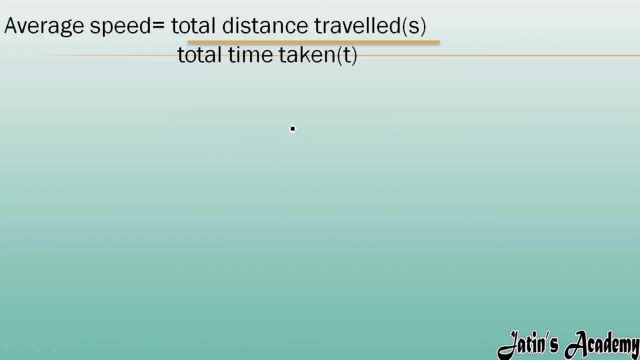 changing of the distance and different time taken. Okay, So we will do one numerical also related to this. So example: first: we are having an athlete covered a distance of 100 meter in 10 seconds. So athlete covered distance of 100 meter. So here we are, given with distance, Distance, we have given 100 meter, Time given. 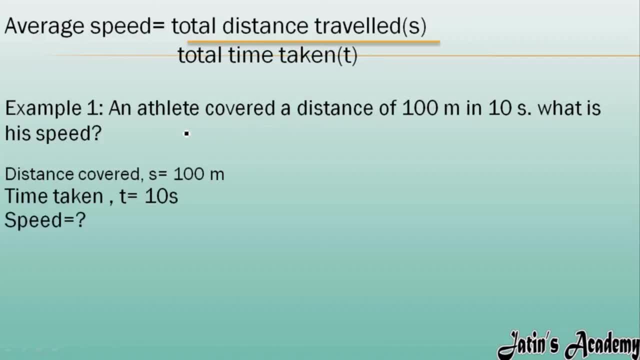 is time taken is given that is 10 seconds. So, simply, we have to calculate the speed. So might be, as you are, knowing what is the formula for speed, Speed formula. Speed formula is: speed is equals to distance over time, Distance travelled over total time taken. 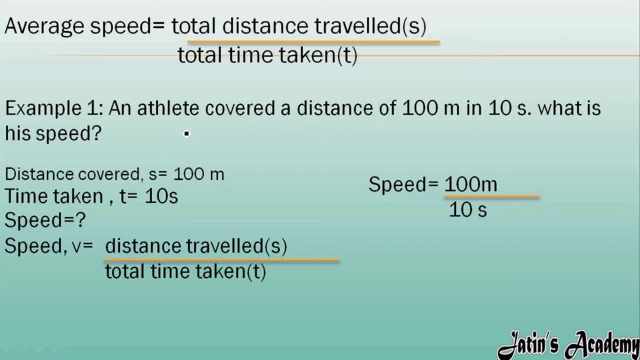 So what do you mean by distance over time? Distance is given to us 100 meter. What is the time given? 10 second. So simply solve it. it will give you 10 meter per second. This is 0. you can cut with this 0. So it is 10 meter per second as a speed. Next we 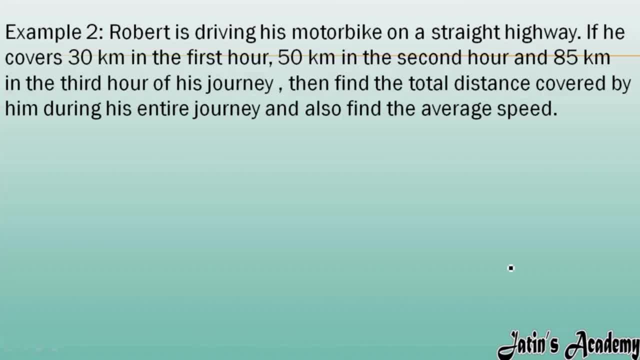 are having. Robert is driving his motorbike on a straight highway. so one robber name is there, one boy is there who is driving his motorbike on a straight highway if he covers 30 kilometer in first hour. so what do you mean by what is given to us? 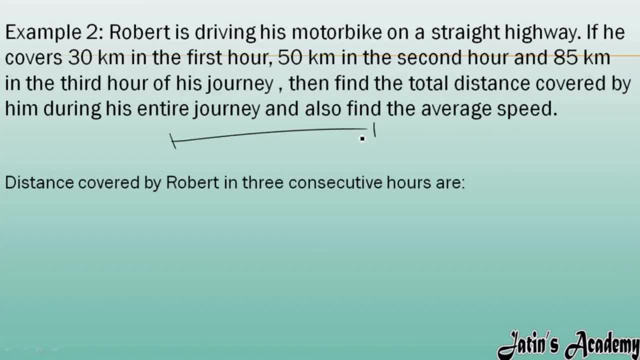 first 30 kilometer, for example, just straight road. in first hour he is covering 30 kilometer, then in the second hour, again in one hour, he is covering 50 kilometer, then again in one hour. in third hour he is covering 85 kilometer. actually, it is given to us.